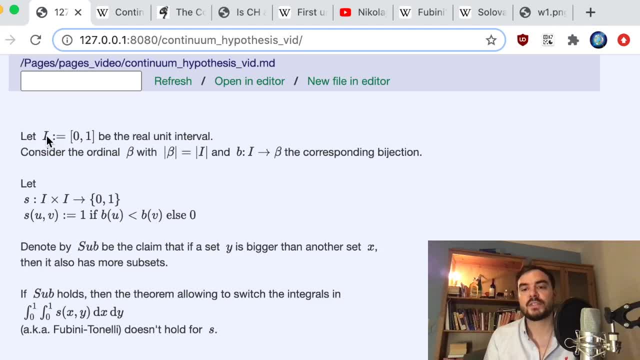 smaller than two thirds. But now we are going to consider another set, beta, which is of the same size. then our real unit unit interval. right, the real unit interval. It is an uncountable set. it actually has the same cardinality as the real numbers. 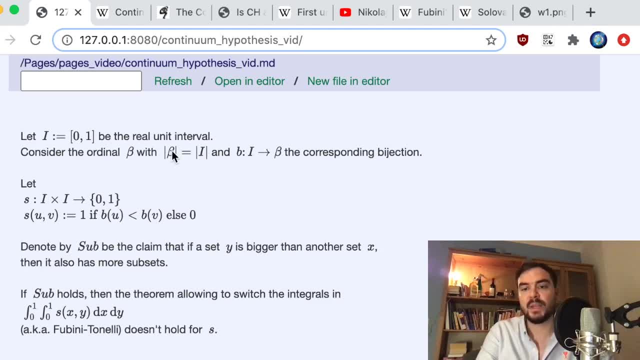 So we're going to consider and set beta, which also has the size of the real numbers. We have here actually a bijection into it and you know, to grant the existence of these functions. we are in the standard foundational framework. Let's say it's Emilio-Fraenkel. 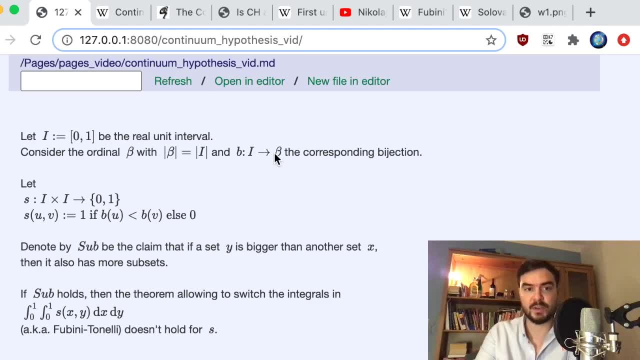 and we're going to use assumed choice, axiom of choice whenever necessary And this, the set beta, is an ordinal, so there is a well-ordered relation on this uncountable set beta. So there is the smallest element in beta and then all the elements in beta can be compared with each other in this, with this. 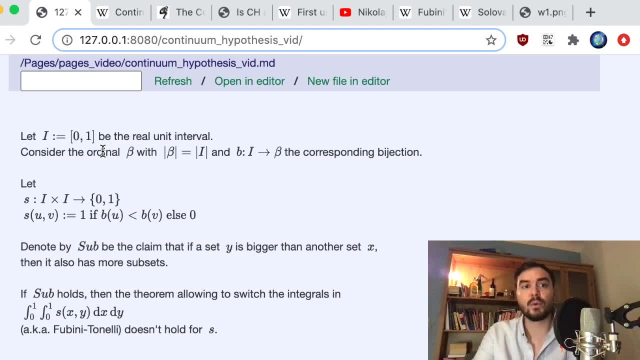 well-ordered relationship. You can think of the von Neumann ordinals if you want. Okay, and now we're going to define a boolean valued function. that is basically just this predicate, but, you know, pulled back to the unit interval. So s is a function from the pairs of real numbers in the interval. 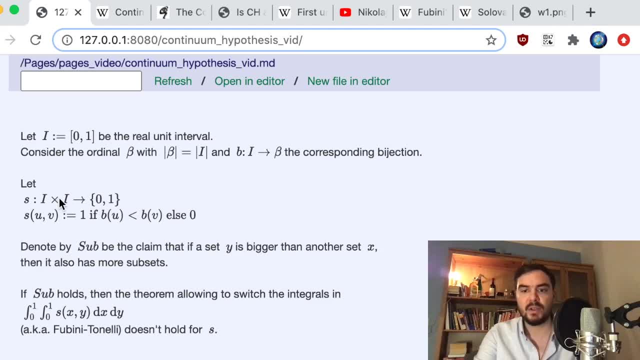 right. you can think of: i times i as the box and the inputs to s are any point in the box and the function returns zero or one, and it is defined as follows: s of u and v is one or true if u is smaller than v, with respect not to the numerical ordering on the in the interval. 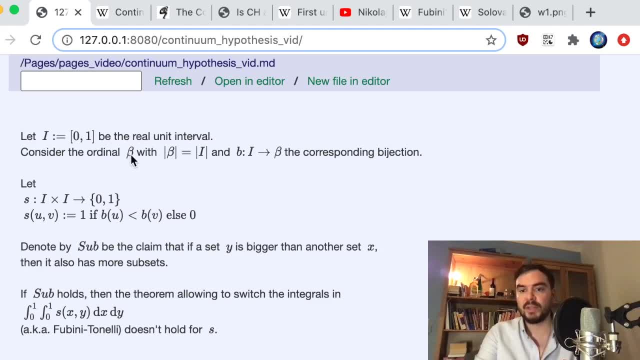 but with respect to the ordering on beta actually, and zero or false, otherwise right. So s is a characteristic function. it really just represents this is small than claim. so that's why i call it s, because it's basically smaller, but smaller not with respect to the. 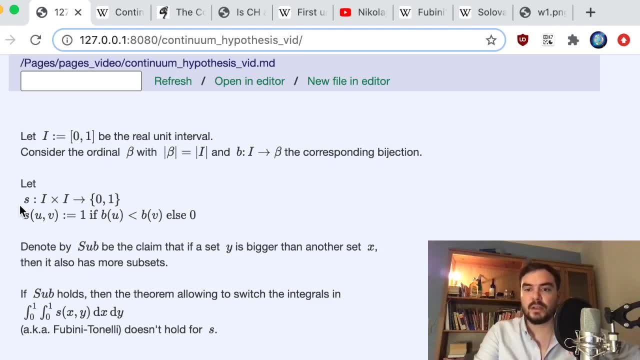 numerical ordering that everybody is familiar with, but with the ordering that is fixed by this bijection b. right b basically determines which real values are bigger than each other. so for example, of course in the real numbers one half is smaller than two thirds. But if this projection kind of flips these, the numbers around, like the numbers, the correspondences around, then it could be that because B is such that then number two thirds is smaller than one half with respect to the ordering on B. 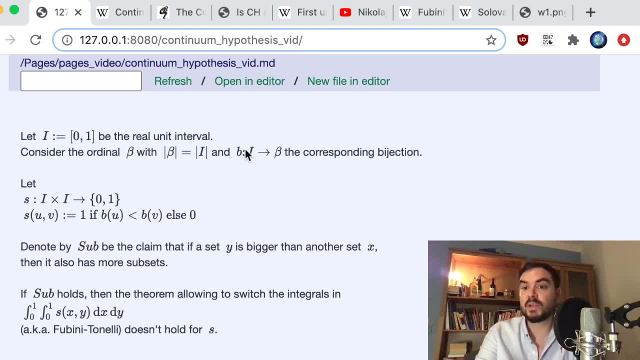 So this B, this small beta, so this B is really just a reordering of the real numbers, if you will here, But a well-ordering, Okay, So, yeah, Okay. And now something which sounds unrelated, right. 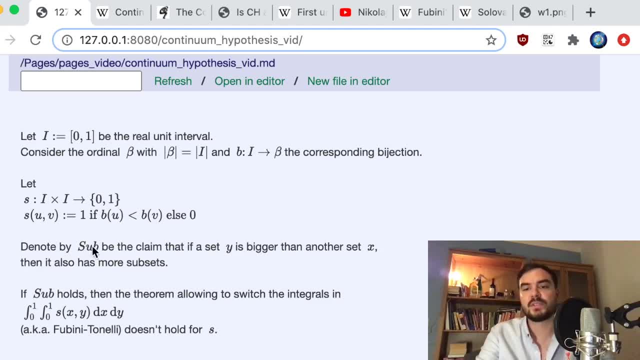 So denote by sub- this is the name for this proposition- the following claim: If a set Y is bigger than another set X, then Y also has more subsets than X. Okay, Sounds real. Reasonable enough. Okay, But now the following. 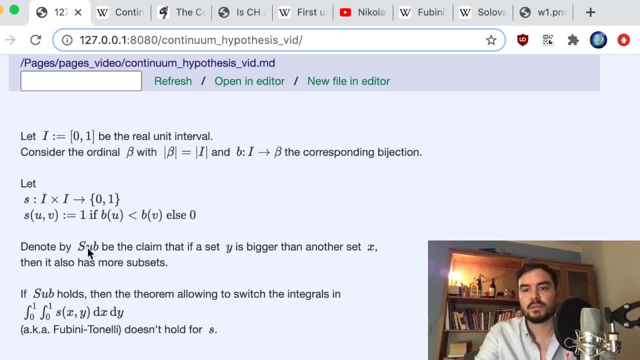 If this proposition sub holds right, If let's say we assume it's true, then the theorem allowing for the integrals to be switched around, you know, in measure theory or integration theory or analysis, doesn't actually hold for this S. 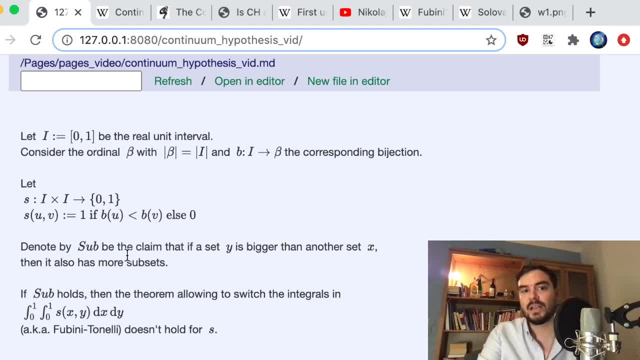 If we allow this, like if we are allowed, assume this, This claim, if you assume it's true, then it follows that actually this: the integrals can not be changed, And I can give you more information. It's because S ceases to be measurable. 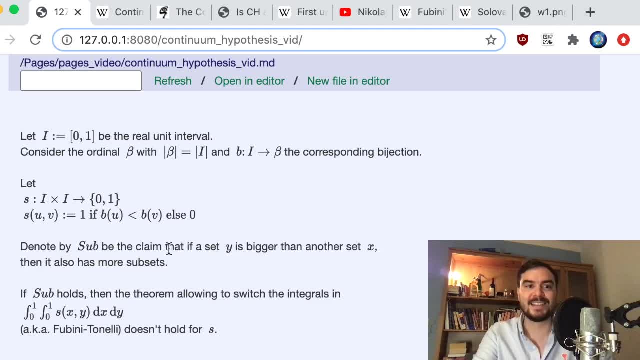 So somehow, somehow, this claim has impact on the measurability of this function. S Okay, Curious enough. Okay, Now I will actually take this a step back and talk about Different, similar, set theoretic questions that then lead up to the continuum hypothesis in a more modern formulation. 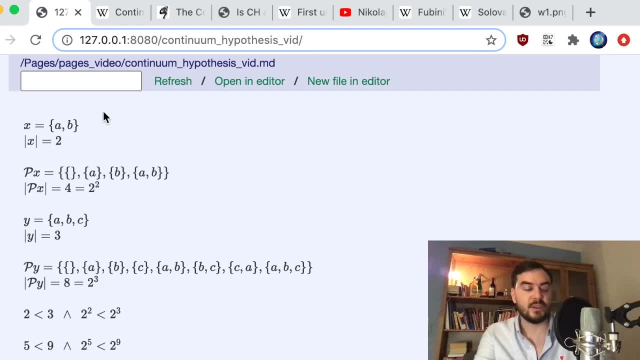 Okay, So this is super, super like elementary. Let's say we have a set. It has two generic elements. you know, in Timmie-Loh-Fraenkel theory theory these elements will also be subsets. Um, we write, um, we use this notation to say X is two elements. 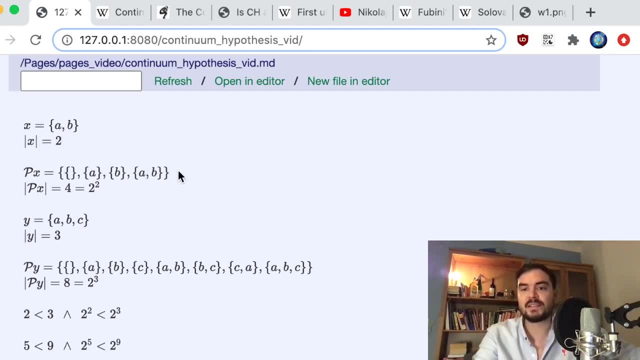 Okay, And then we can compute the subsets And again, in this classical framework, we can easily find: oh, these are the subsets. Um then, how many subsets that this X actually have? Well, we can count. we find this: four. four happens to be two to the power of two. 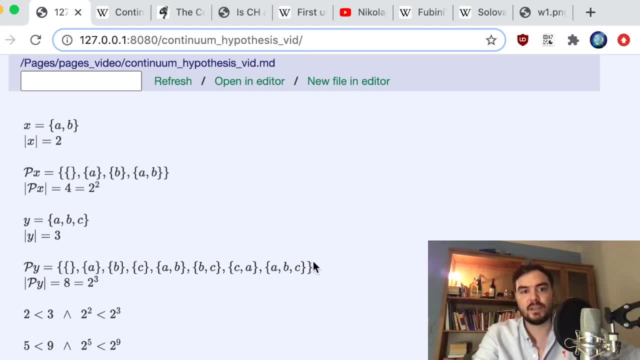 If you do the same with this three element set, we can find the number of subsets. We find it's eight, it's two to the power of three And you might know the number of sets, subsets of an N element set if it's finite. 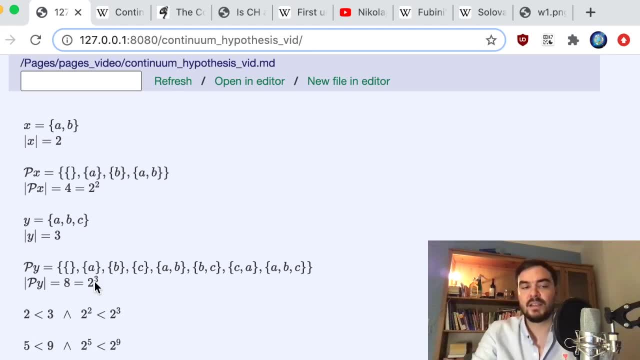 And if you Using classical logic, then this is two to the power of the size of the set. So here's standard observation. This is really like, just evident, like two is smaller than three, Yeah, And also two to the power of two is smaller than two to the power of three, or five is smaller than nine. 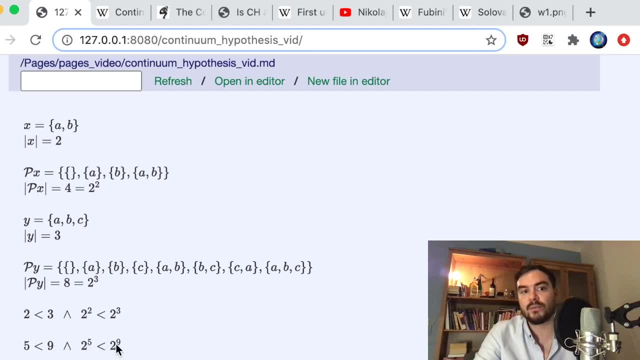 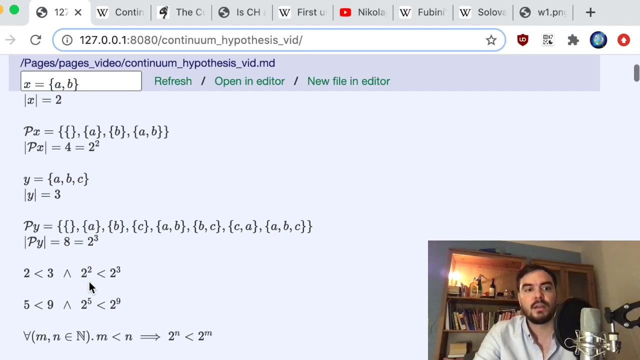 And two to the power of five is smaller than two to the power of nine. So, okay, We have- uh, these are arithmetic claims- We Either the power set, the size of the power set is given by a two to the power of the size of the um the set and and uh, cardinal wise, this um remains. 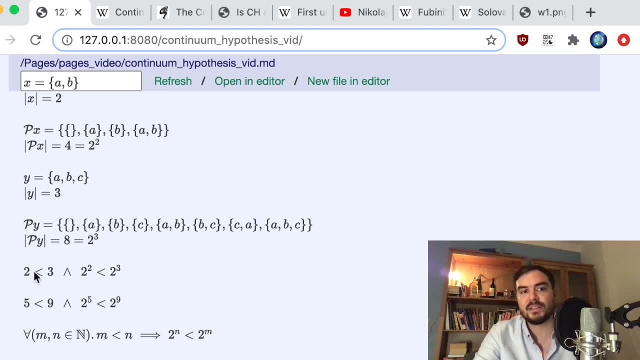 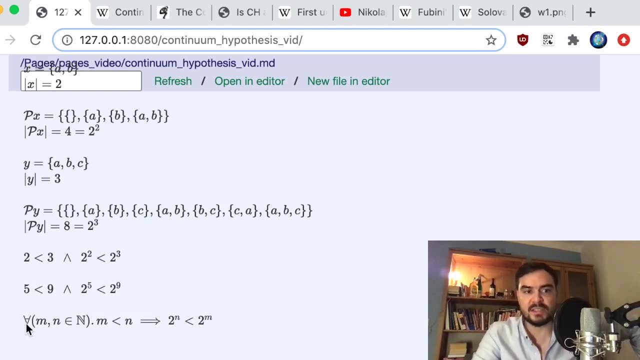 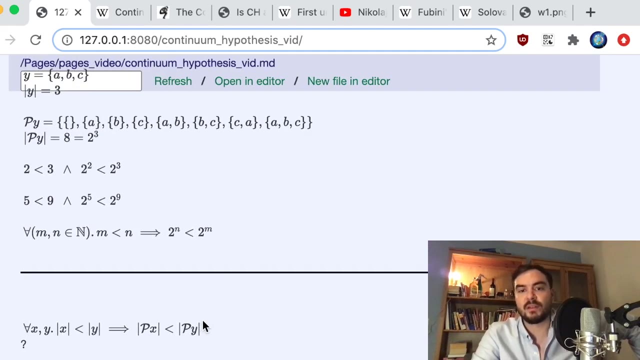 So then the question is: does this this uh order, uh relations? um, will they hold? uh, will it really hold, like for D? this is a statement about the natural numbers. No, this is pretty clear. Um, but now, if you pass on to the sort of set, theoretical foundation here, this is exactly this uh statement, except now we're considering general sets. 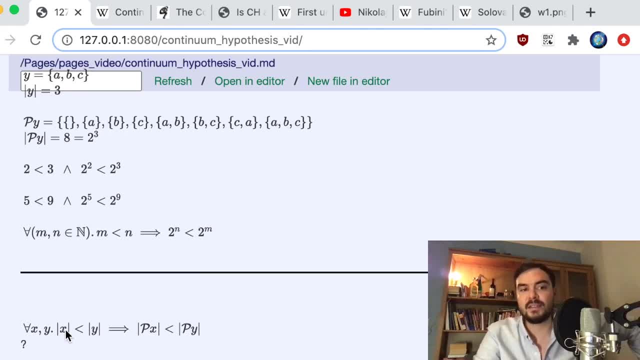 They can also be infinite. Um, and this is the statement that I asked before. So if a set X is smaller than a set Y, does that mean it has also less subsets? You can think about it. You can think about to prove it here. 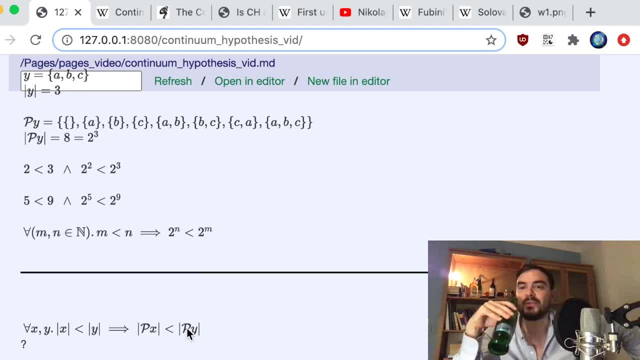 I give you, I give you three seconds to think about a good proof for that. Well, it will depend on. to depend on your axiom set, of course, Right, But the funny thing is that this statement is actually independent of the Milo Franklin choice. 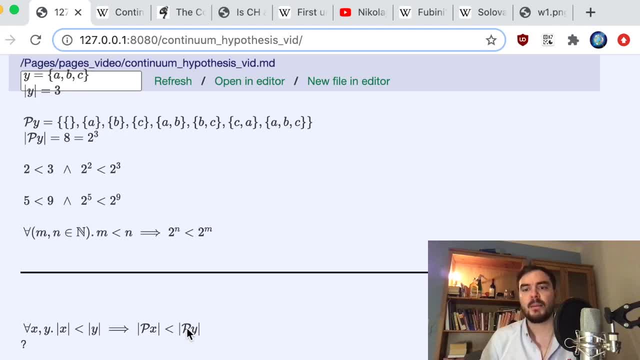 So it looks very elementary, Um, but you can use a lot of very strong um uh, set theoretical axioms and you can actually use much stronger, like large cardinal accents and whatnot. Uh, you will not be able to actually prove this, interestingly enough, from these axioms. 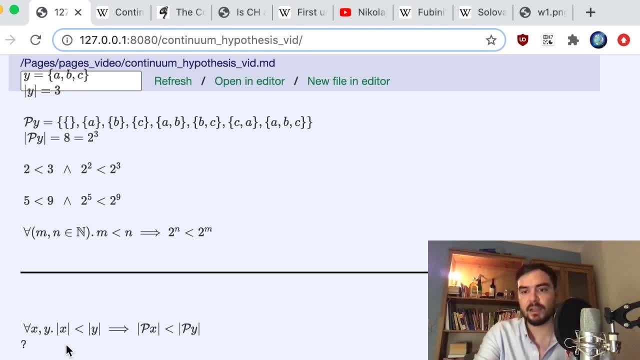 Okay, Um, but okay, Uh. this is uh like, for example: I think this is a direct consequence, then, of the generalized continuum hypothesis, but let's go on, uh, to the actual continuum hypothesis, Right, Uh, which is a little bit more concrete than that. 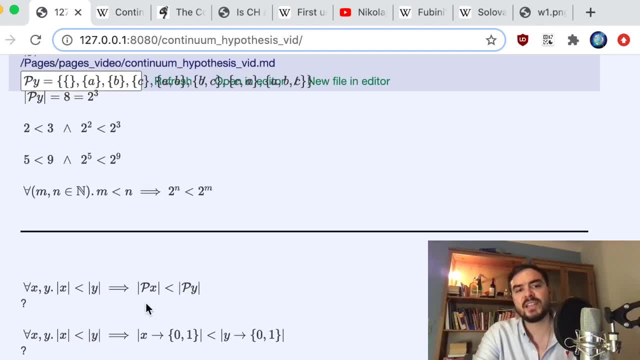 So yeah, um, here's a uh restatement. I talked about the number of subsets. I can also like talk about the number of co characteristic functions. right, The functions from the set into this two element set classically. 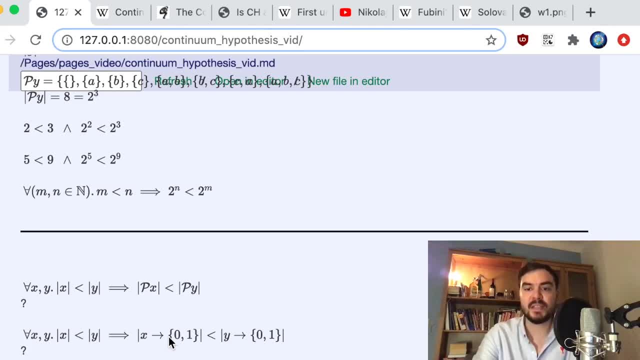 This will be, um, exactly the same statement, essentially, um, constructively characteristic functions are a little bit, quite a bit, uh, simpler to handle. then subsets: subsets which, uh, you know, corresponds to the fact that subsets are attained with by the separation axiom. but okay, let's not get into a constructive set theory yet. 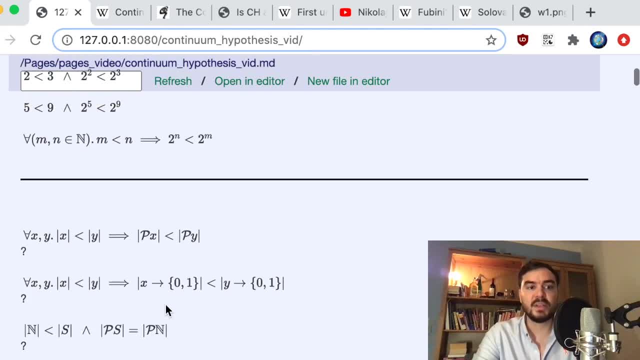 Um, maybe in another video, but here I will. uh, sorry, I will. I will make some more statements and you can think about them. Okay, So here is a conjunction. Is it possible, Let me ask like that: Is it possible that you have a set S which is smaller than the uh, which is bigger than the natural numbers, a set S which is bigger than the set of natural numbers, but the number of subsets and the size of the power sets is the same? 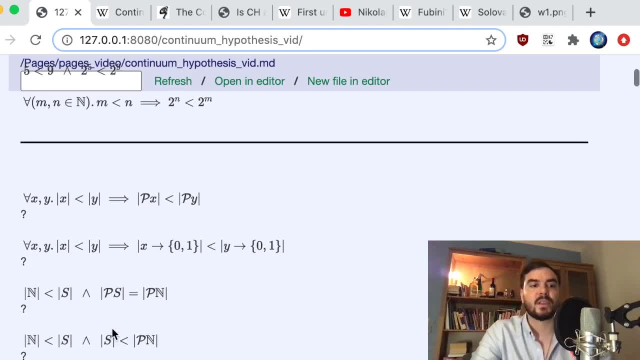 Is it possible? Um same condition Is it? Is it possible that you have, uh, a set which is bigger than the natural numbers and the set is smaller than the number of subsets of the natural numbers? right, This is essentially, uh, an early version of the continuum hypothesis, here even more concrete, right? 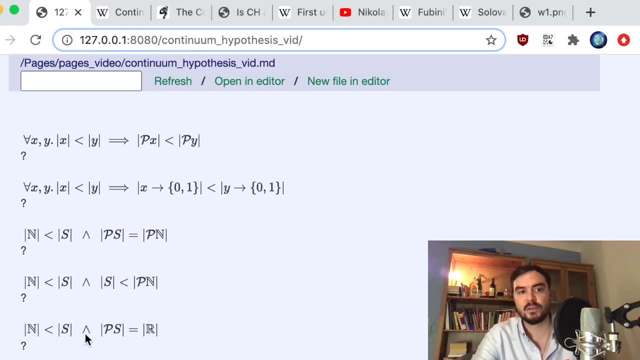 The, the power set of the national numbers corresponds also to the real. So, Uh, this is a variant of this, of that statement here: um, where uh like already replaced the P of N, I I like to say the number of. uh, you know, I I like to see the class of subsets of the natural numbers which, because this is the one of the most easiest ways to to define it- 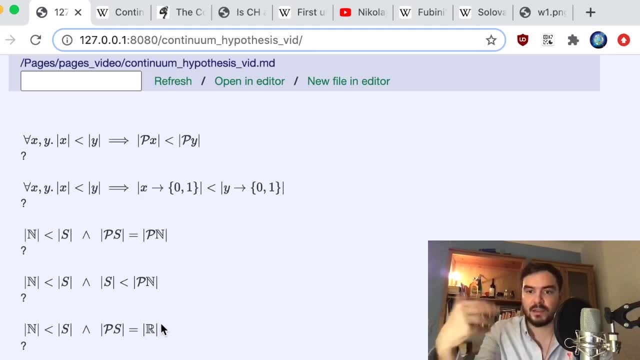 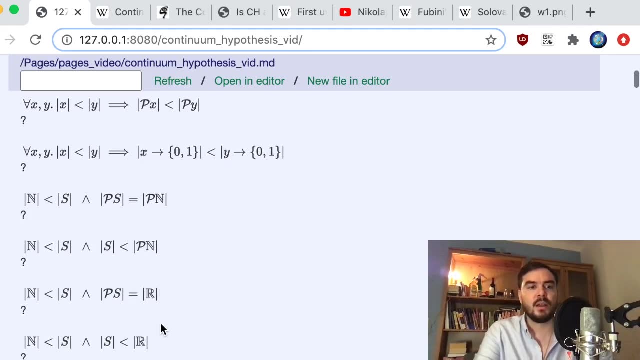 Um, but you can just say the real numbers, right, If you like. uh know about all the these correspondences And they have the right axioms to set it up. Um, yeah, And here here's the same. this is the statement with the reals replaced. 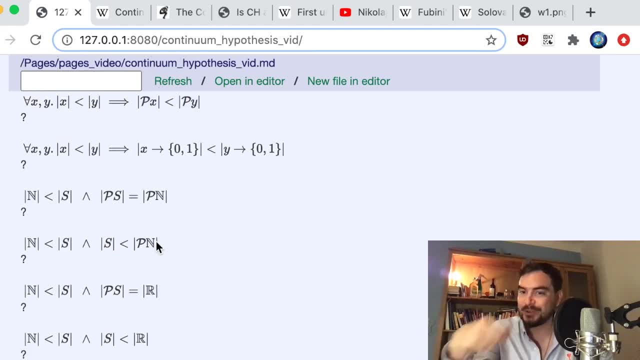 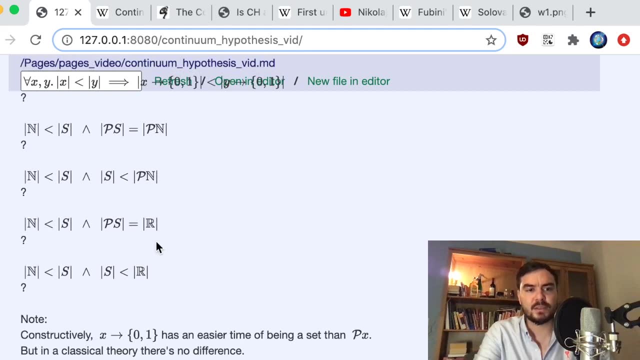 Uh. so these are all all uh like interesting questions. You can ponder a little bit about them. Um, now go on. Yeah, I make some uh remarks, So, as I already said, uh characteristic functions a little bit easier to handle uh constructively. 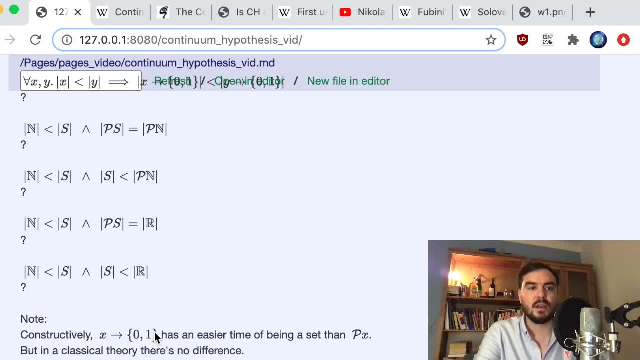 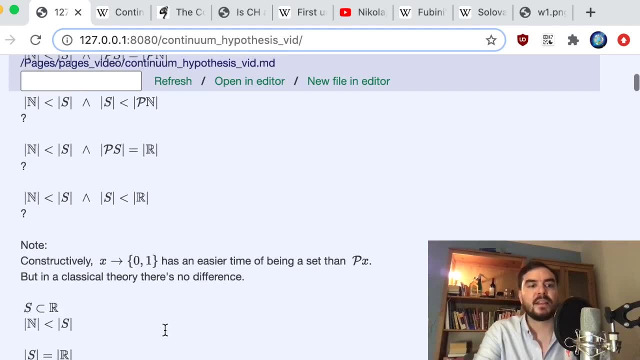 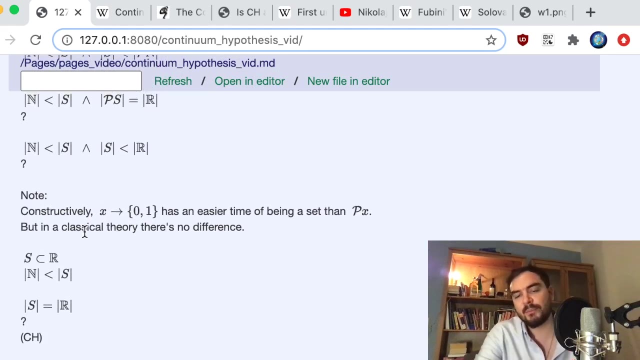 Um, I will get into that in future videos. Um, but in any case, in this case, in this video, we speak about classical theory. This is the same thing. Um and yeah, okay, And now, uh, I just, you know, state a continuum hypothesis in, in, in a form. uh, it's very similar to the one I already stated. 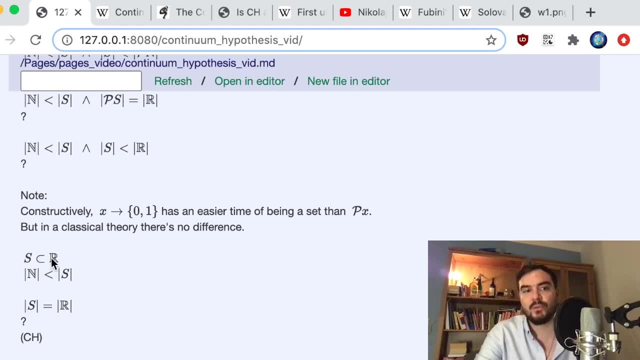 So let S be a subset of the real numbers. This is a generic, a priori, a generic uh, set of real numbers. Uh, let's consider those which are not, Um, uh, finite or countable, right. 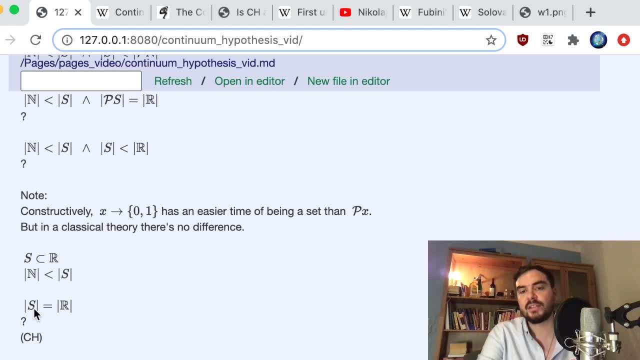 The S shall be bigger. Is it the case that then, this S is just as big as the real numbers? That's a continuum hypothesis. There's a statement which cannot be proven from similar frankly choice. Okay, But there are other uh formulations and this is sort of what we're going to get into before we come back to the integral statement. 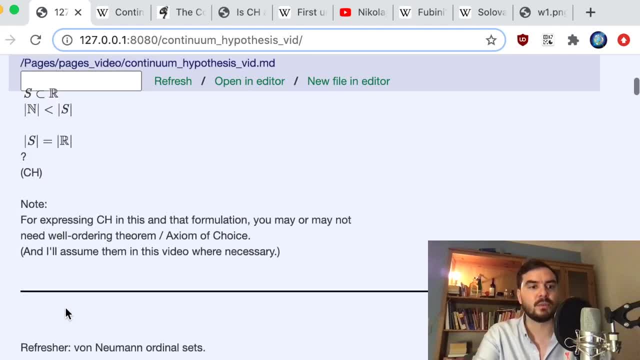 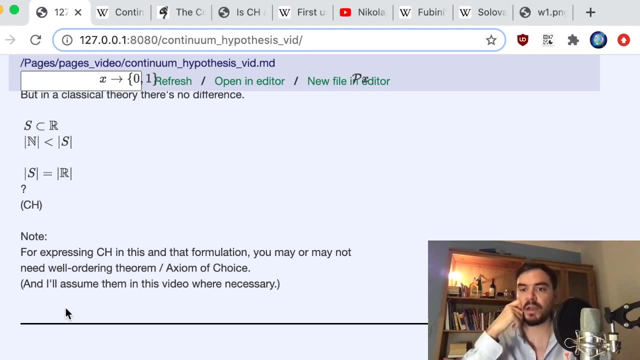 Uh, see why that makes sense. Um okay, What kind of notes do I have here? Um okay, I mentioned it already. Like uh, whenever you demand or there is a projection between these ordinals, these cardinals, then you might have to invoke the axiom of choice. 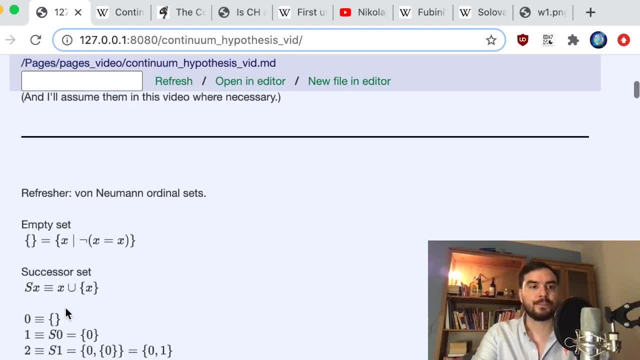 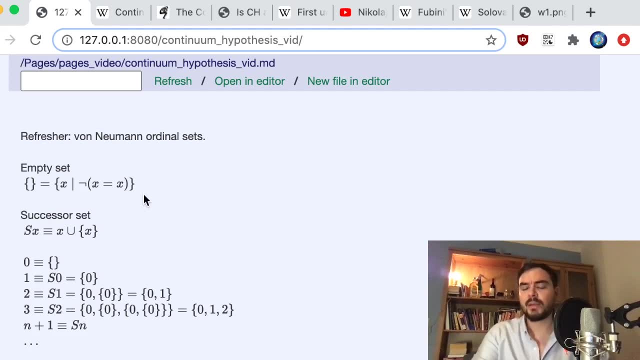 If you want to make these claims, um, good, Uh, let me for a minute talk about, uh, ordinary numbers. So maybe let's make a break here and I will step through this sort of tabs I have open here. Um, because I have talked. 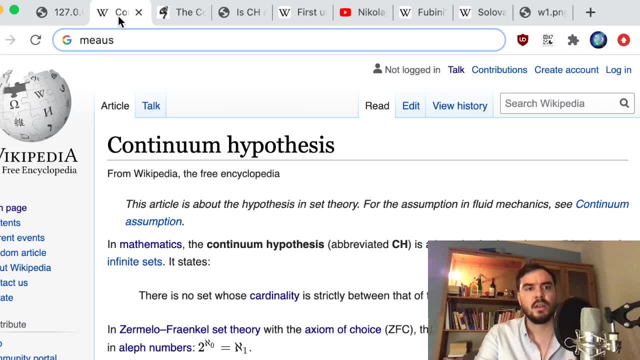 About ordinary numbers a couple of times on this YouTube channel before. uh, these things are the ones you, as always, find the bottom in the uh gist uh Wikipedia article on the continuum hypothesis. uh, then the Stanford encyclopedia article on it. 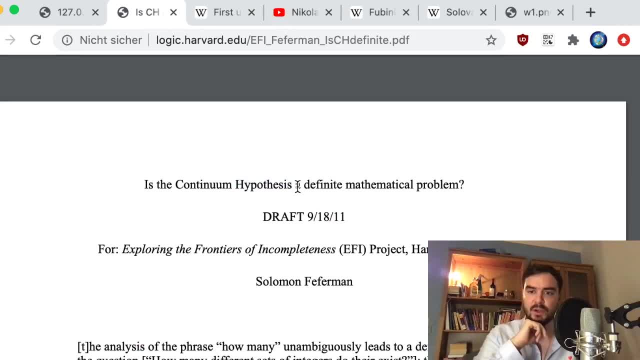 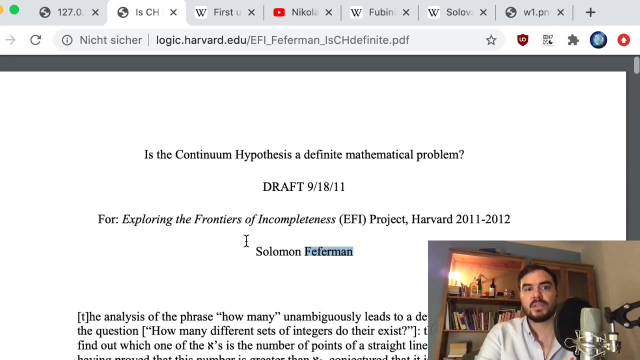 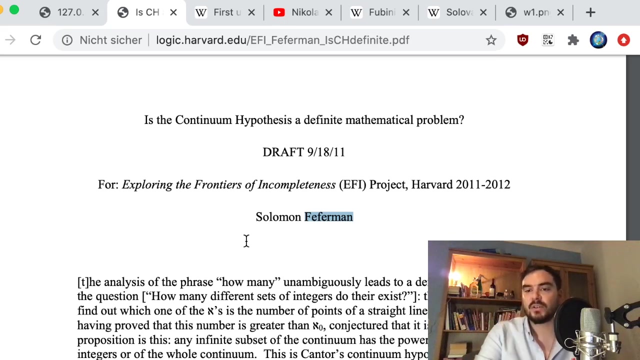 Um. in my impredicativity video a month ago or two I talked about papers by Fefferman, who does did constructive theory. Some Certainly knows what's up in set fear as well. He has an interesting uh perspective and in this paper lays it out. and the paper is nice because it also has various reformulations in terms of different um axioms. 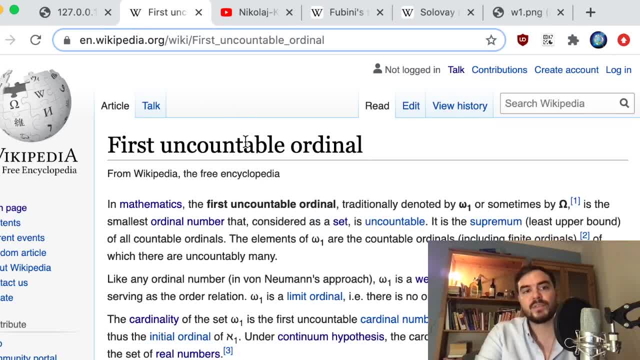 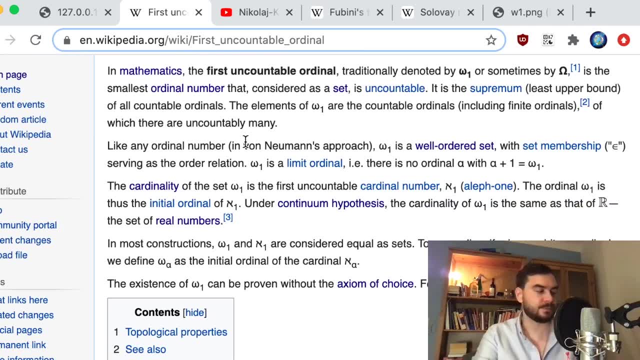 Uh, what's going to be relevant in the remainder of this video is the first uncountable ordinal, So you may uh quickly skim that here. I will mention it anyway in a second. Um, But uh, this is just in omega one, the first ordinal you can think of phenomenon ordinals, which has the size of the reels. 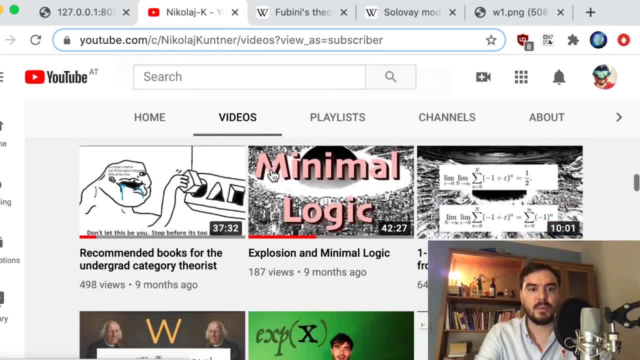 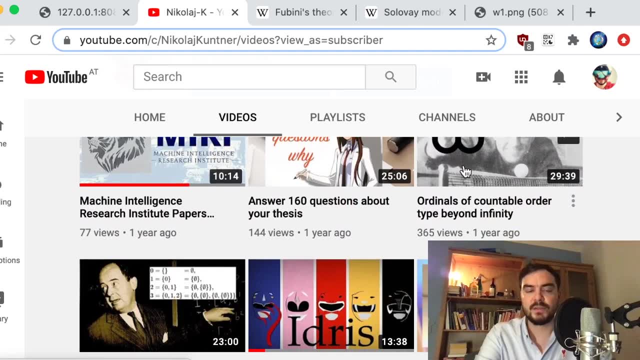 Okay, Um so on, uh, my YouTube channel. I talked about, uh, all the numbers before. I think I motivated them more or less well here in this video where I describe omega uh square to countable ordinal omega squared. 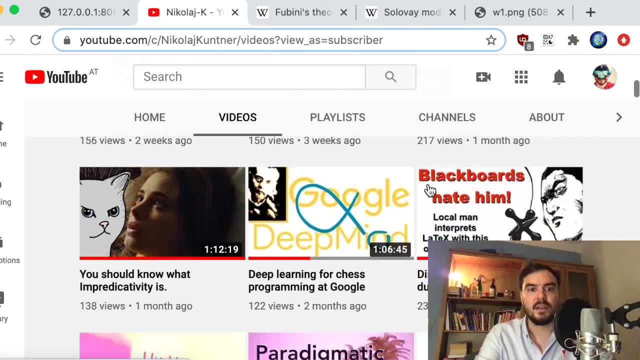 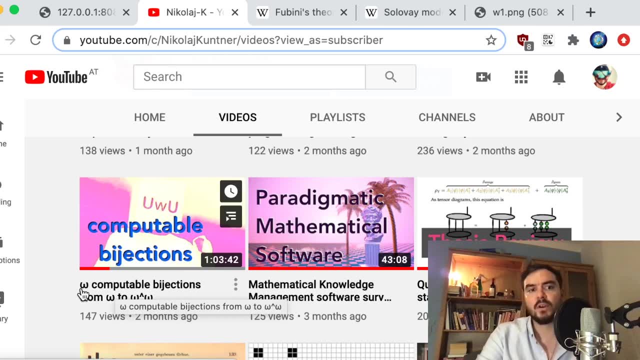 And then there is This um nice bijection between, uh, relatively large, uh, countable ordinal here, where I map bijectively omega to omega to the omega. This is, um, well, the null exponentiation. Um, these are the videos related where I in detail, in more detail, explain the ordinals, right? 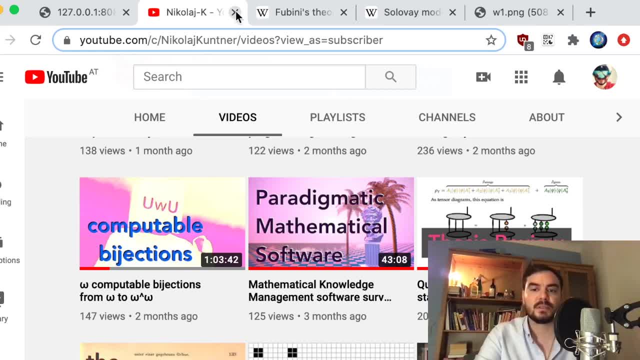 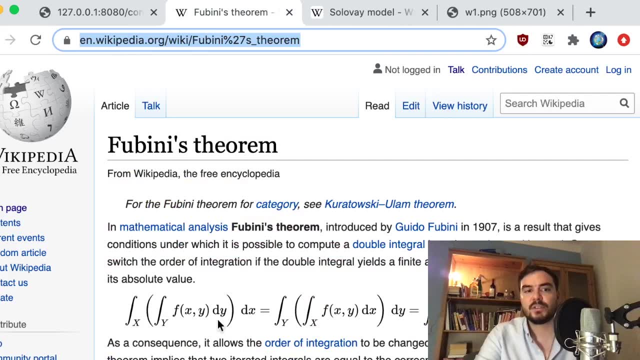 Um, I'm going to quickly summarize it in a second. but um, you might, uh, If you're interested in that, look into that. Okay, For Pini's theorem, you know just that you can switch that uh integral, uh integrals there. 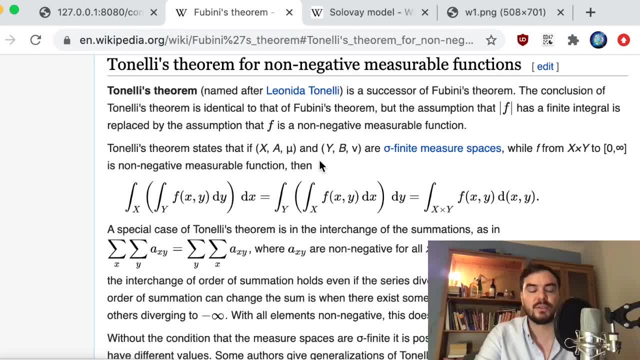 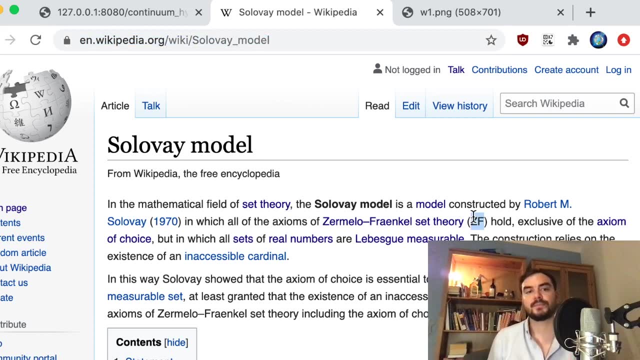 And of course, they add on various reformulations. The one that's most relevant in this video is the Tonelli formulation: uh, where it speaks about measurable functions, because that's what we're going to break Um. and then interesting is: uh, in the middle of ankle there is um, there is models where 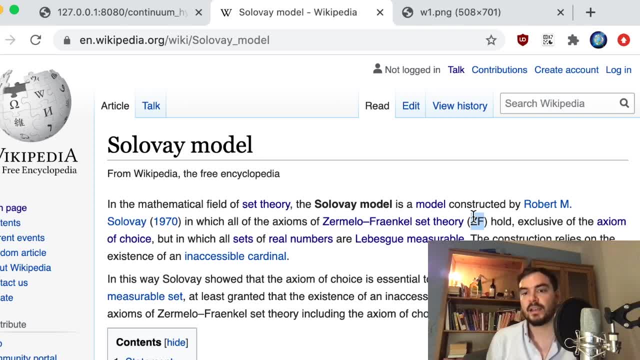 Everything Is measurable, right, That uh excludes the axiom of choice, because that implies uh existence of non-measurable functions, given giving rise um to the famous, some some of the famous paradoxes in set theory, um tasky paradox and so on. 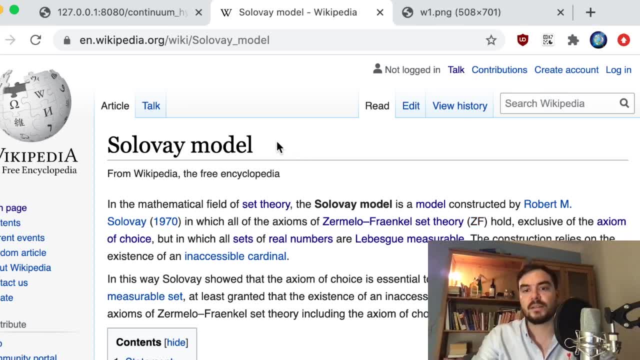 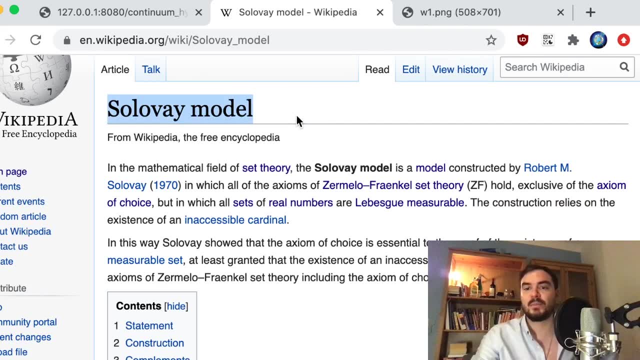 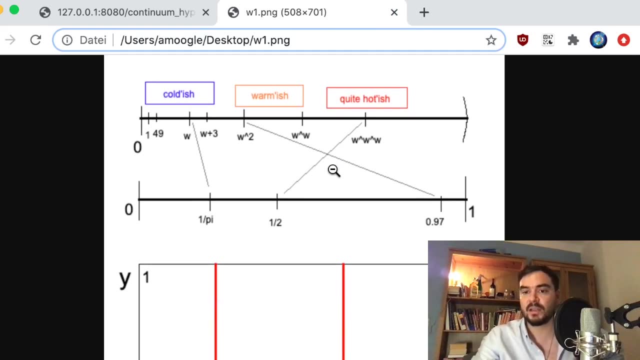 Um and also uh. this model rejects the continuum hypothesis, as we will demonstrate in this video, Because the continuum hypothesis implies the existence of non-measurable functions. Uh, and then, finally, I have this uh picture here that I will uh, that I will use to motivate the proof that we're going to see. 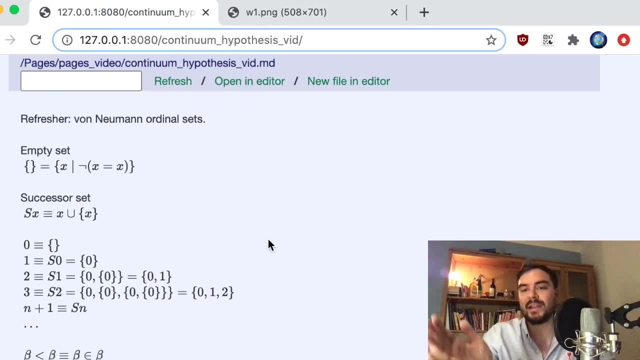 Okay, So, uh, refresher, I quickly explain the von Neumann ordinals, because the first uncountable ordinal, in that sense will be relevant. So we define the empty set: right At a visage, there's just an empty set, which, which is a set which has: 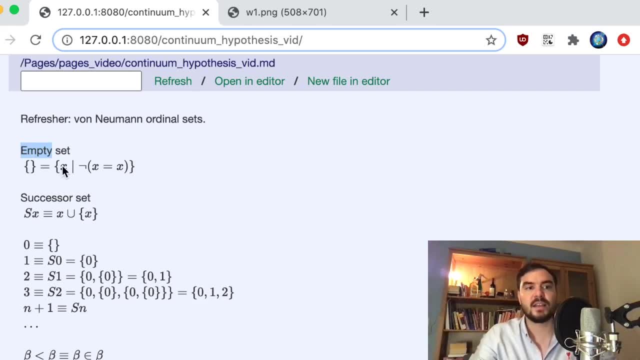 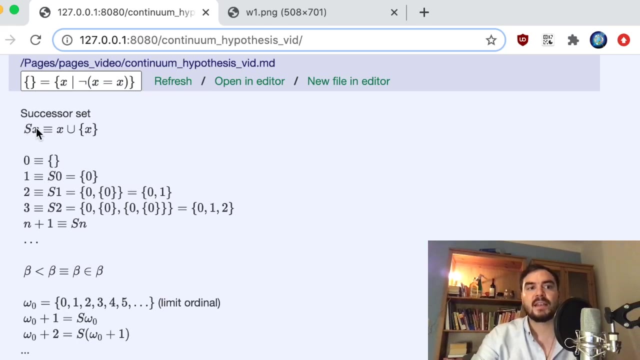 No elements. or we say we define the empty set as the set of all elements, um for which uh false statement holds. This is an example of a false statement. So this is a set which has no elements. This success operation, uh S, X, means just the union of X and the singleton where X is in it. 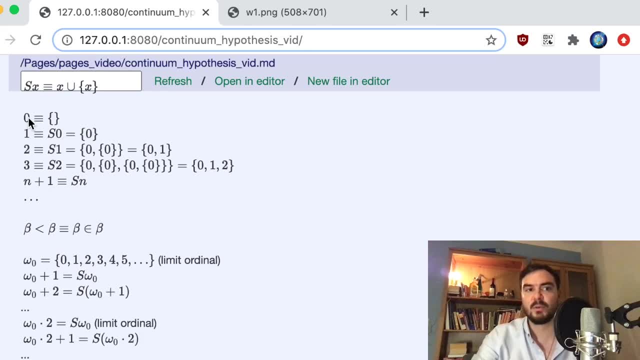 And in this way we can define natural numbers right. The zero which has mean the empty set. Uh, one, It's the success of zero- turns out to be the set which has exactly one element. Two is the success of one which turns out is exactly this element, with the set with two elements, and so on and so forth. 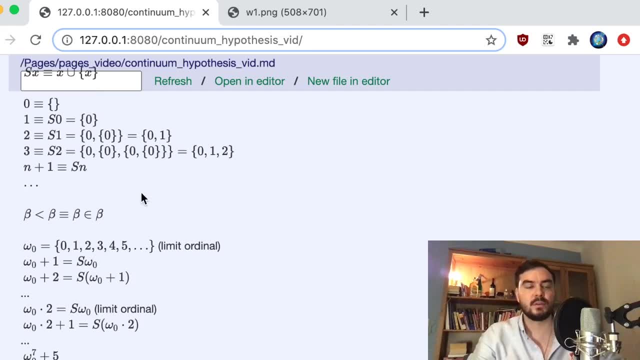 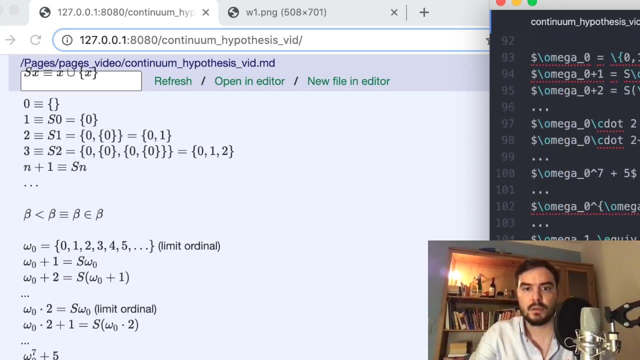 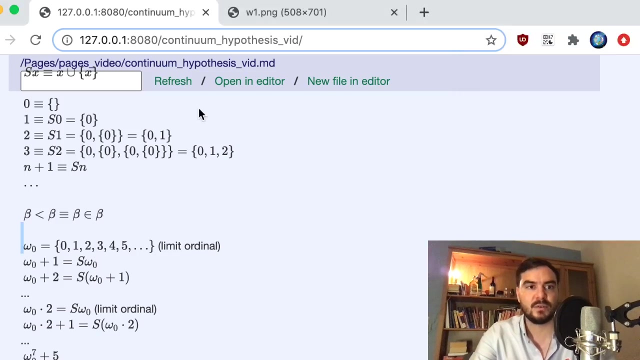 Um, sorry, there is a typo here with a minute Um, namely: uh, this smaller relation is not what I want. I can correct it. Um, this happened because I I used uh search and replace functions to find good letters. 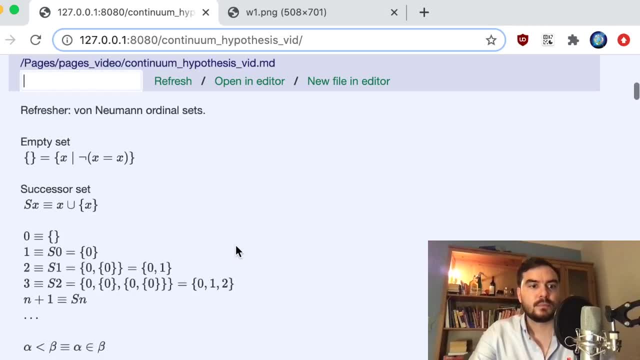 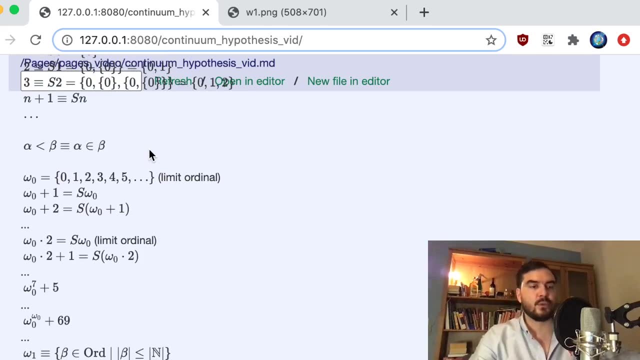 Hmm, Okay, And so, um for this, for this, uh, when I'm an ordinance, we define um these, the relation smaller than uh, just by this element, relation that we see the set free has, uh, these elements in it. 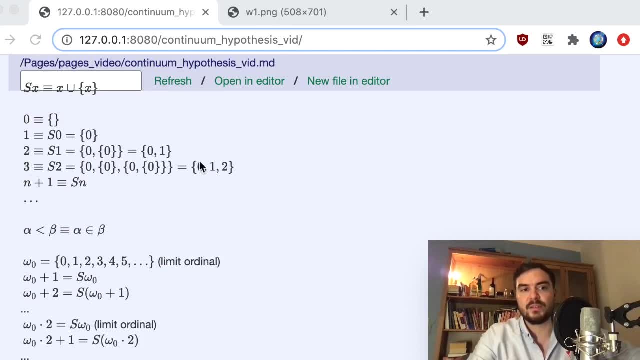 And one is smaller than three is represented very nicely by the fact that one is member of three right. This just works out in the phenomenon ordinance Um, and then we can not just do the success operation but we can also from limit ordinance by um this collecting operations, where we take anything. 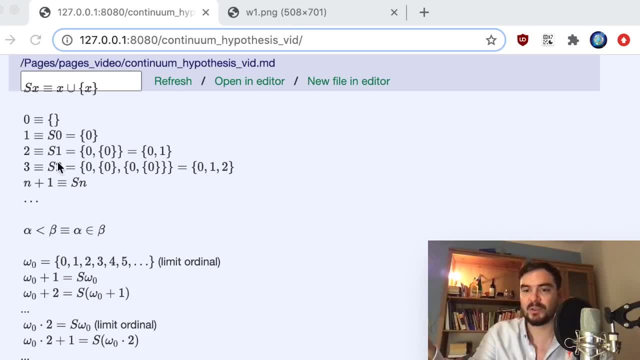 So we take, we like, Uh, I don't talk about, uh set, theoretical induction, uh, here about taking all these, these very finite objects and putting them all into one set gives an infinite set, uh, Omega zero, which has all the natural numbers in it. 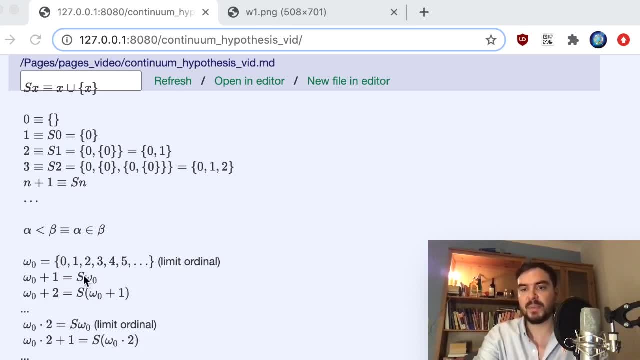 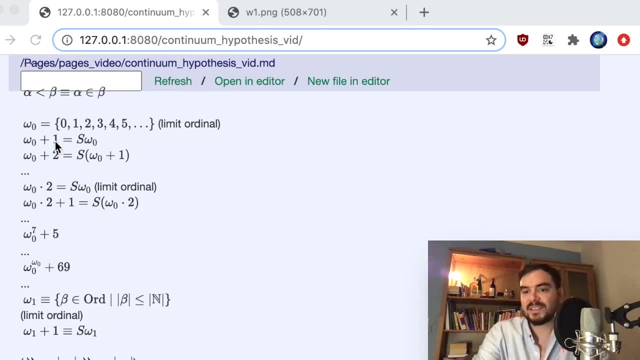 And then we have that. but the success operation is still a basic set, theoretical operation that we can do on any set. So we can do, uh, Omega zero plus one, right, This is just a set. when you can see, there's the second infinite set. 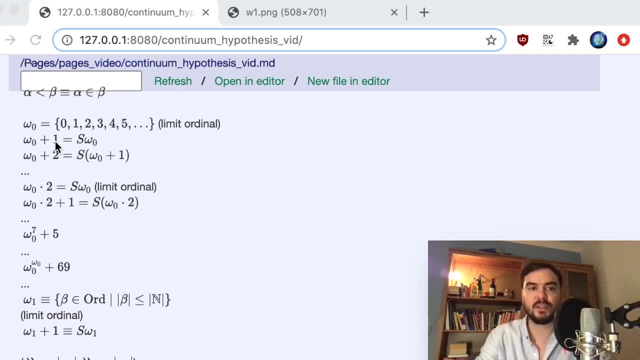 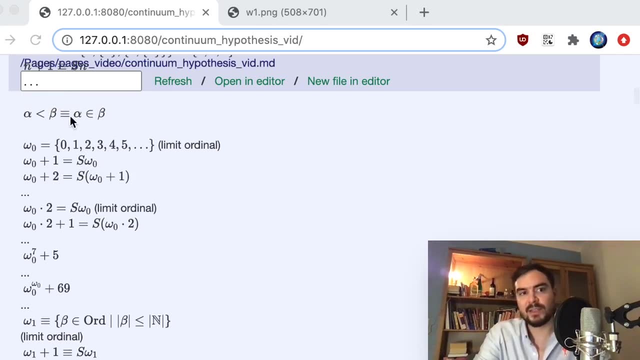 Um, but uh, there's not even necessarily. we just consider it here. As I said, we don't have to make any of these associations. Um, but the ordering is very nicely here. It's still defined, Okay, And, and so this goes on. we can define uh on a arithmetic and all. 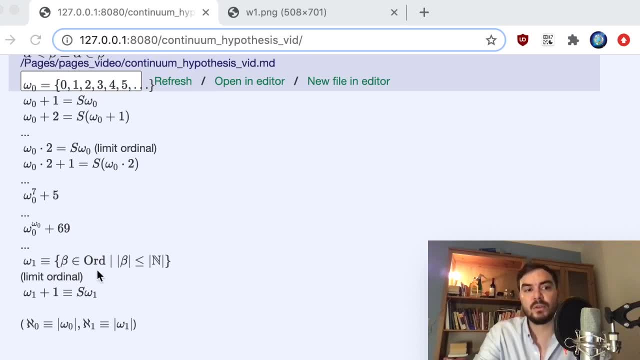 Okay, And eventually, um, if, uh, you let me write here like we can define what is an ordinary, this, this, uh, transitive, um structure that I just defined, And um, so We can define the class of ordinals and we say, uh, we can then go on and define, uh, Omega one, which is what we want to get at. 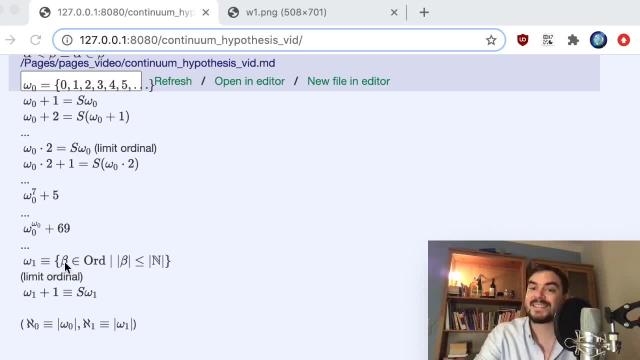 So Omega one is all the uh ordinals, all the sets which are ordinals- This is what this represents here- Um which are uh finite or accountable right. So Omega one is a set that has all the uh finite or accountable ordinals and this limit all the uh happens. 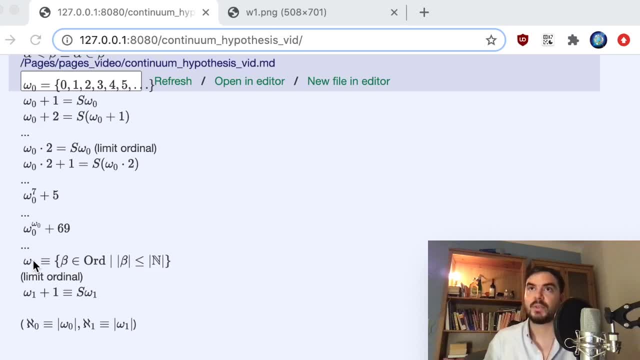 To be um happens to be uncountable. So this is basically the. you can think of it as the small, smallest uncountable set, Right, Um. so if, in case, you make the mistake in your head and think about the real numbers as the smallest um uncountable set, well then you assume the continuum hypothesis already. 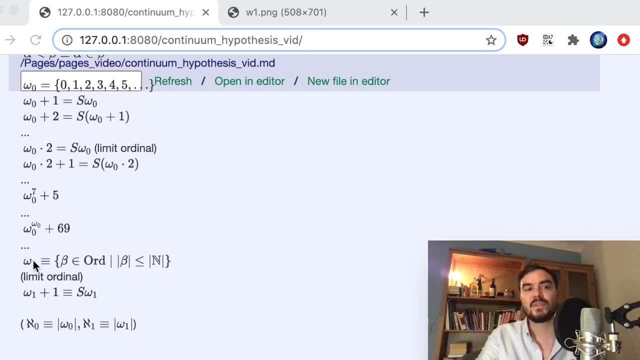 This is wrong thinking. Let's say um, uh Here, uh, from like you need to assume less and get to this nice, nice set. You don't have to define any like real arithmetic, um to get to this uncountable set. 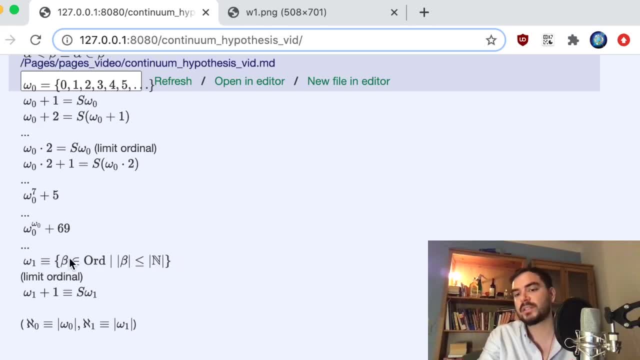 And uh, since you had, these ordinals represent all the types. um you, you don't get lower than that, And of course, you can also go on. Now you can say: well, what is the second uncountable ordinal? 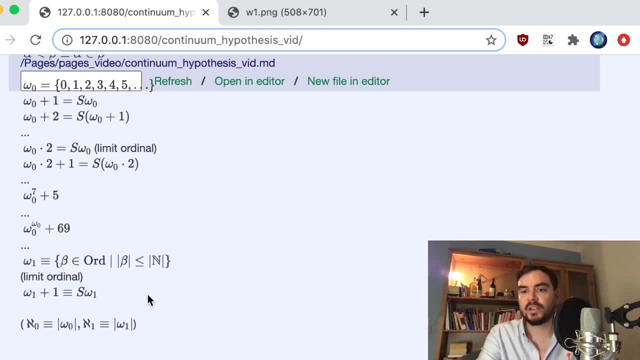 Well, it's just a success of that, But We're not interested in ordinals which are larger in this, uh, this sense that omega one. we're interested in omega one and we might introduce these notations: right, I'll have zero and a phone. 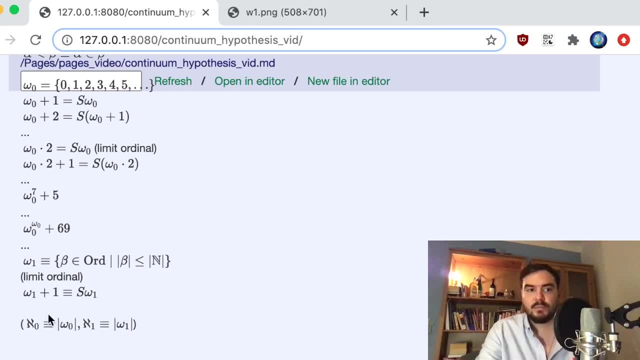 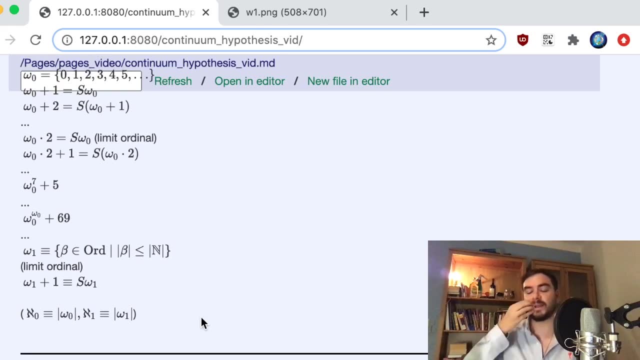 I'm not going to use RF notation in the video. What is basically just? it's basically just that it's just notation. Um, and there's also like another ups, like a more abstract theory about of ordinals. You don't have to squeeze everything into similar Franklin set theory and define. 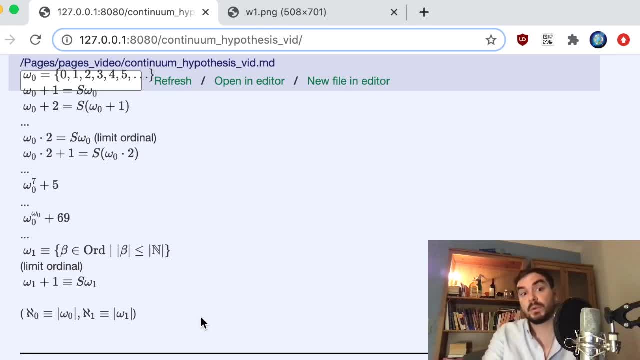 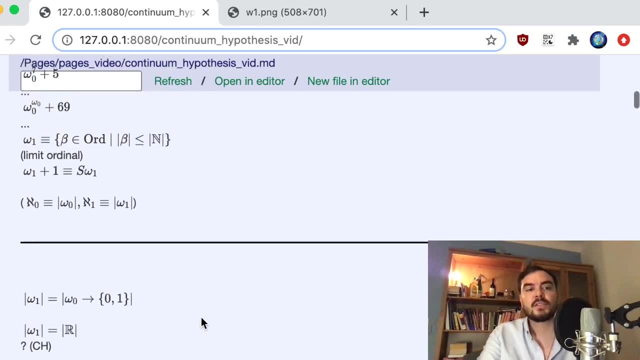 Things like that, but it's possible. Um, that's, that's what we are going to go here with this. uh, representation by Von Neumann. Okay, And um, so, uh, with this we have this formulation right. 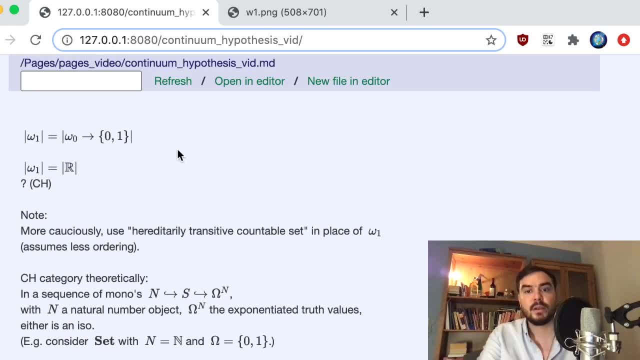 Um, can I go there without spoiling? Yeah, Okay. So if omega one, if you think of it as the smallest, um uncountable, set um, then we can ask these questions: uh, is this Small, small, the smallest? it's omega one, the smallest, uncountable? uh, ordinal, uh, is it's cardinality? 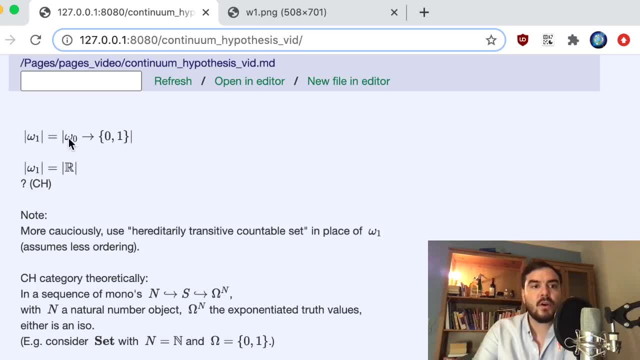 Meaning? is it in projection to uh, the map of uh all characteristic functions for omega one from basically the natural numbers into a two element set right Or state the differently classically is the size of uh omega one The? 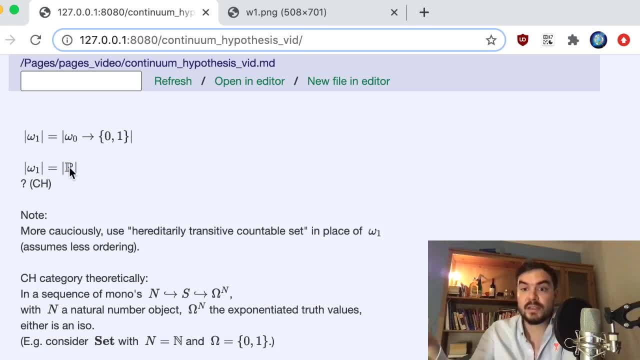 Same size as that of the reels, In other words is. in other words, the continuing hypothesis says: are the reels actually a quite small set? Like, of course, the reels are big, they're an uncountable set, whatever big means. but the continuum hypothesis is that actually the reels or the, the, the size of the class of the subsets of the natural numbers or the size of this characteristic functions is as small as it could possibly be. 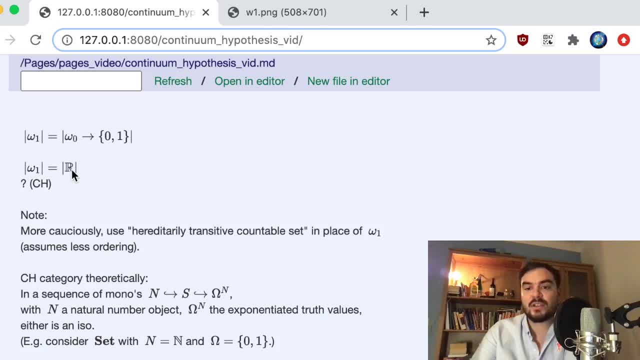 Right, Right, Right Right. So if this is true, then R is actually, you know, it's kind of, it's kind of uh, squeezed like at the very bottom of what it could be, that's that's step offices. 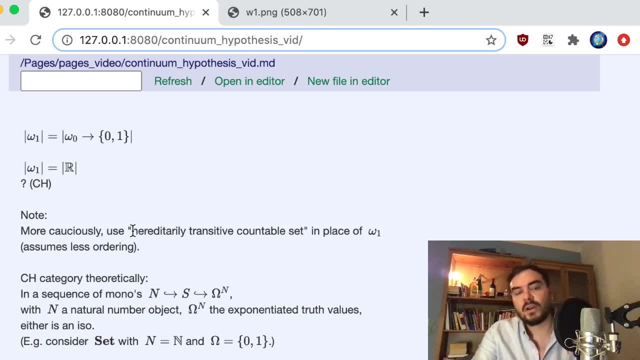 Okay, Um, yeah. so since, like, I'm shilling constructive uh logic a little bit on the channel, if you want to not assume too much about orderings- and this gets harder in a constructive setting like ordering things and making decisions- 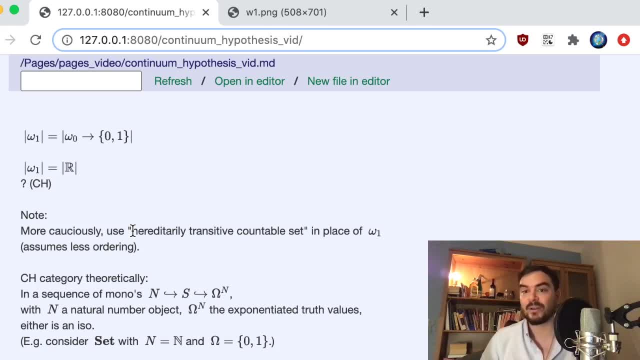 For example, if you hear you know uh questions about um, uh ordering, deciding or uh ordering, then we can just say the hereditarily trans, uh sensitive accountable sets, Uh, the set of these sets. 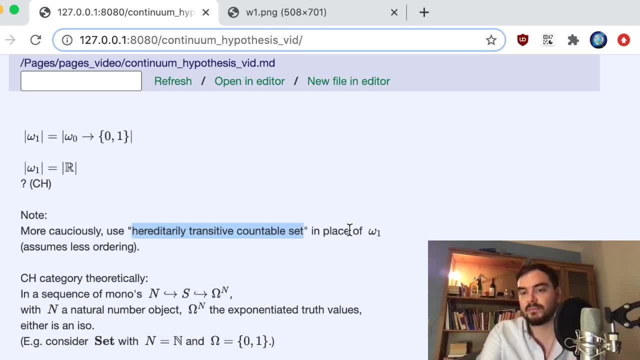 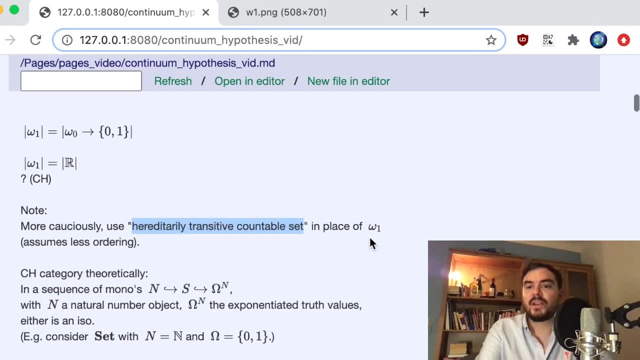 Um, and then we have something, the classical equivalent to what I've just defined here: Um, and also, like we can, we can put this, the statement, in a more categorical era: theoretic setting right, Uh huh, We can say: given a sequence of monos or injections, 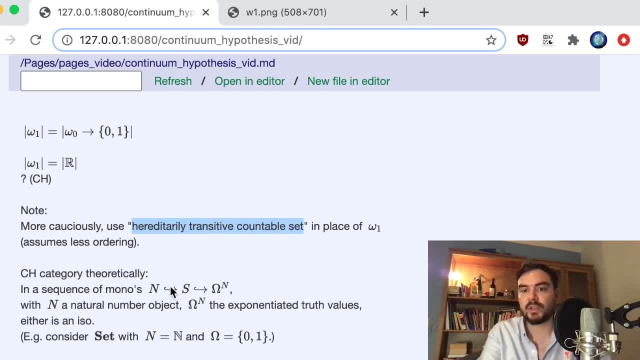 which I denote with this arrow here. there's also other ways of denoting injections, like graphically: So n injects into s injects into the exponential object of n with omega, and n is a natural number object, For example in the category of sets. 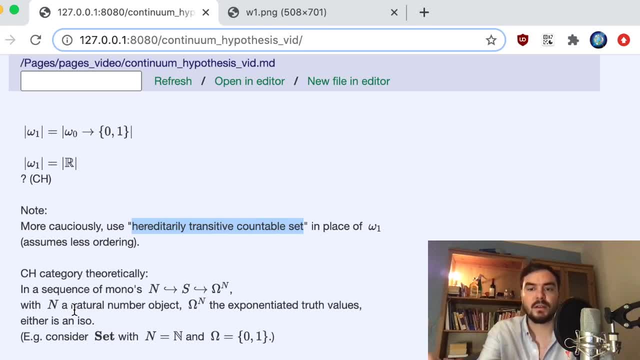 there will be something as big as the omega zero And in topos theory you have this truth, value, object and if it's Cartesian, closed and you can exponentiate it and then get that and you can define monomorphisms very abstractly. 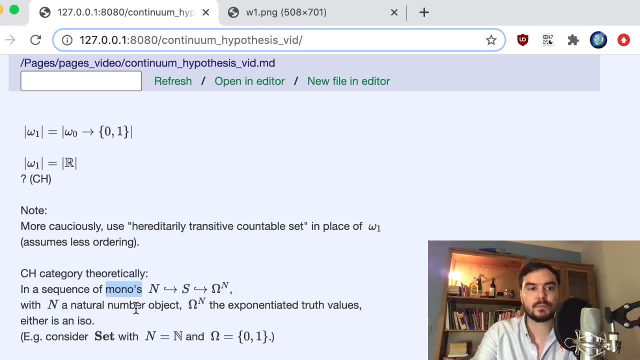 And then the statement is that as soon as you have that, then one of those is actually like an isomorphism. So either this only works because s is actually isomorphic down or because it's isomorphic there. So this is basically: s is like the natural numbers. 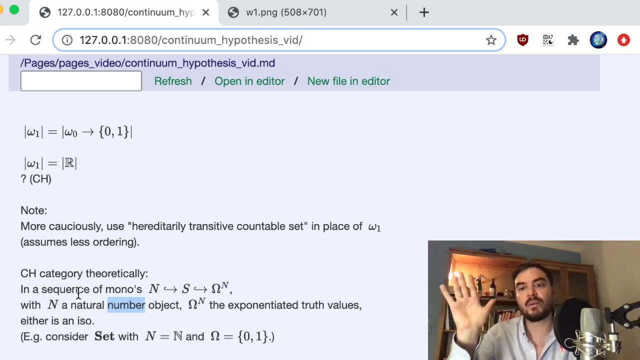 or s is like the real numbers, nothing in between. So this is a purely error theoretical statement. if you're into that, I have not linked it here, but there is this book, Sheaves in Geometry and Logic on topos theory that discusses these sort of perspectives. 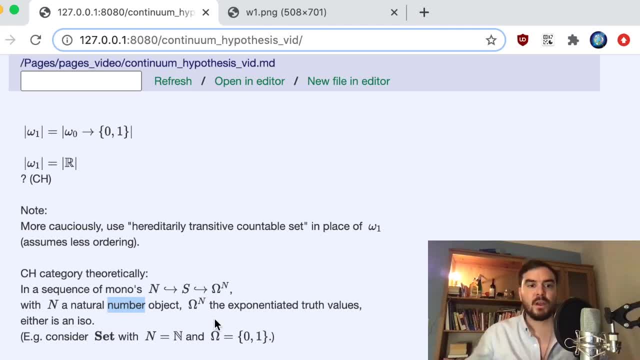 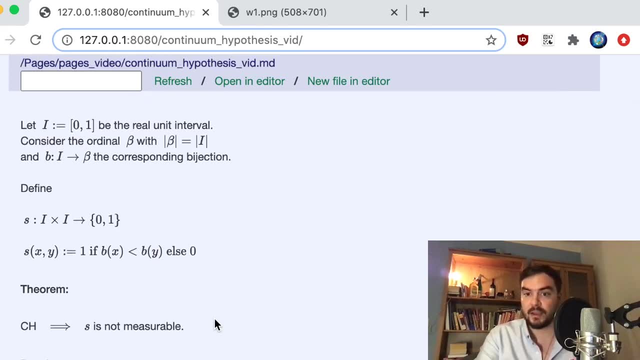 and even discusses perspectives on forcing. Okay, Yeah, and we get to the end. So we are back at the statement, the wild statement, where I said: we have this interval between the numbers between zero and one. Um, we have some ordinal which is in correspondence to that. you know now. 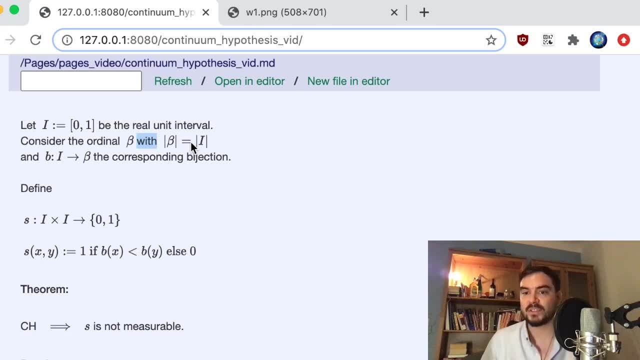 you see, this is basically uh, the continuum hypothesis fixes this. the continuing hypothesis fixes that beta must be the smallest uncountable ordinal omega one. right, The continuum hypothesis is the idea that the real numbers are as small as they could possibly be uncountable, but not too far out. 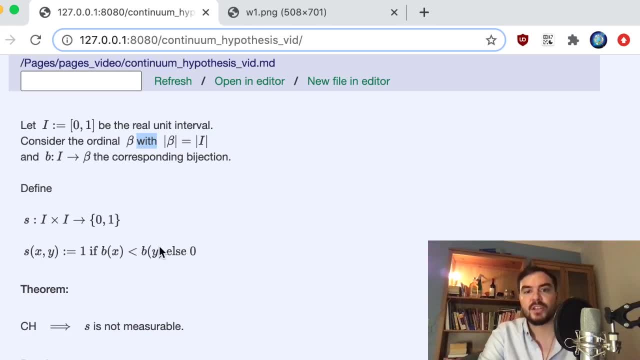 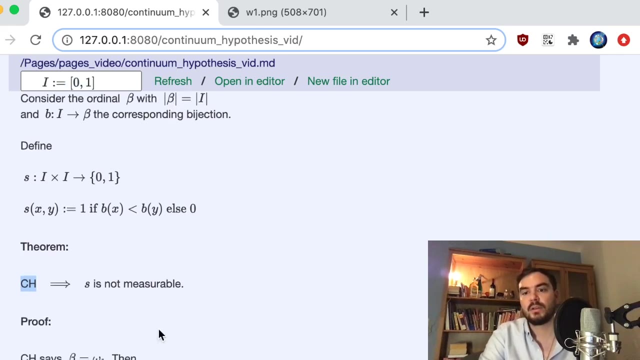 Um, we define the function as before, And then the statement is: if the continuum hypothesis holds, in other words, if beta has the size of omega one, the smallest uncountable ordinal, then S is not measurable. Okay And um, the proof is as follows, and this is almost the end of the video. 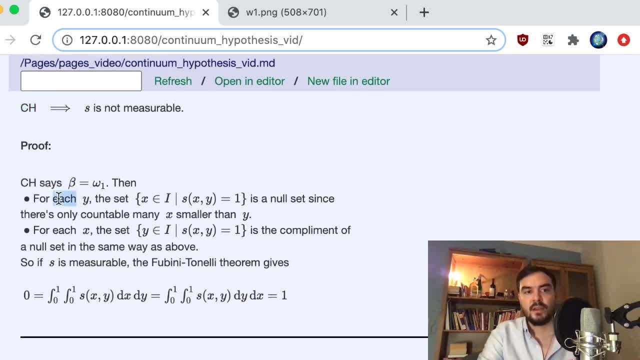 Okay. So, uh, let's say beta is omega one, Then if you fix a Y, Okay, Then the set of all Xs that are smaller with respect to the induced ordering, Um, this is a null set. This is because in an omega one are all the ordinals that are smaller than omega. 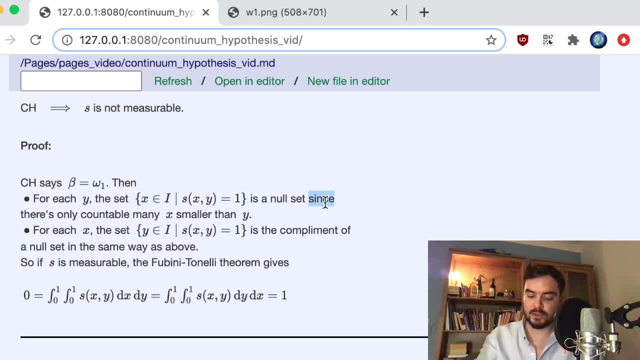 one right by definition: Um and the uh. we set up omega one. We set up the set of all Xs that are smaller than omega one to be the set which holds all the countable ordinals right. 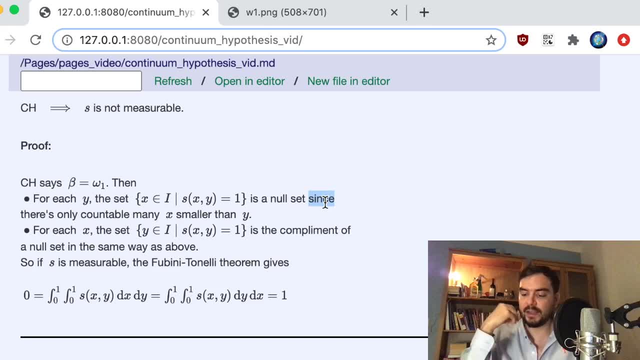 So, whenever you choose any element in omega one, right? Uh, then Then everything below this element you chose can only be countable, right? It can, can, you can only let, you can get there from from below by counting. 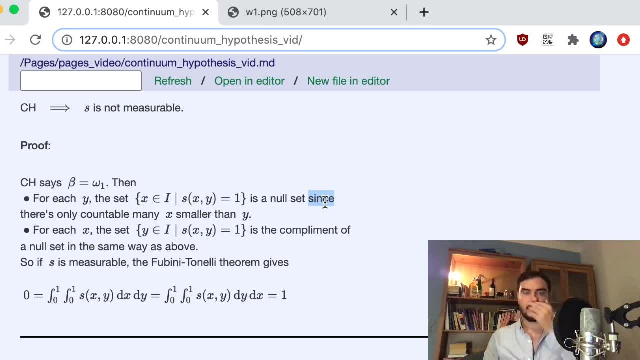 Um, if that makes sense, So I will. I have a picture in a second, Um, but okay, So, uh, I will elaborate in a second, but let's go on Okay Here. Um, similarly, if you fix any X, then all the wise, such that X is smaller than Y, IE, all uh, elements that are bigger than it. 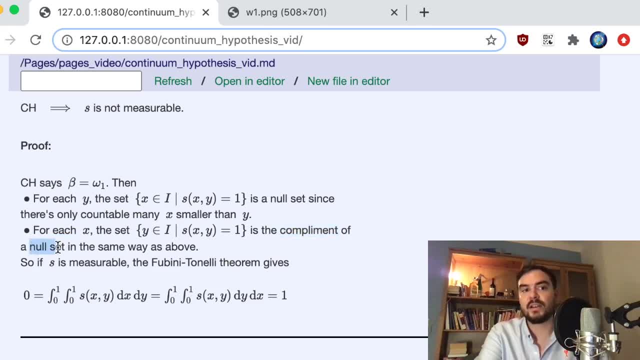 This is the also the compliment of. Okay. So now, uh, null set in uh in um measure, theoretical terms. So again, if you take omega one, take any element, then the set of all ordinals which is above it, this is actually an uncountable set. by the definition of omega one as an uncountable set, 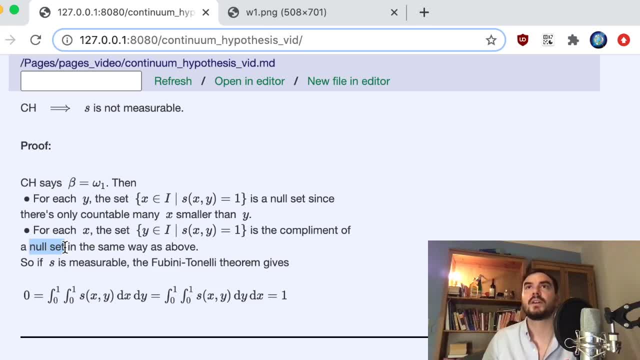 I mean, we have not, we have not proven here that, uh, the set of all So countable set, uh, ordinals, is uncountable, but I suppose you can easily believe it right. So otherwise, you, you can, you can get this set is a member of itself situation. 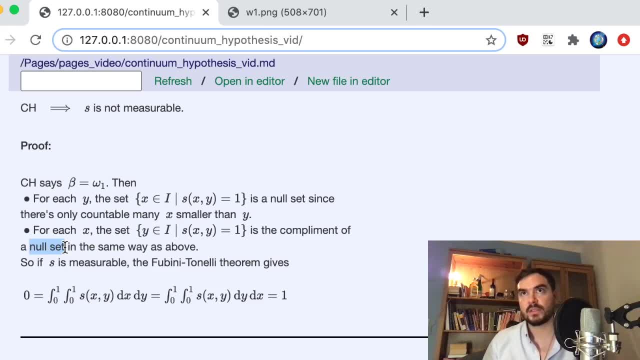 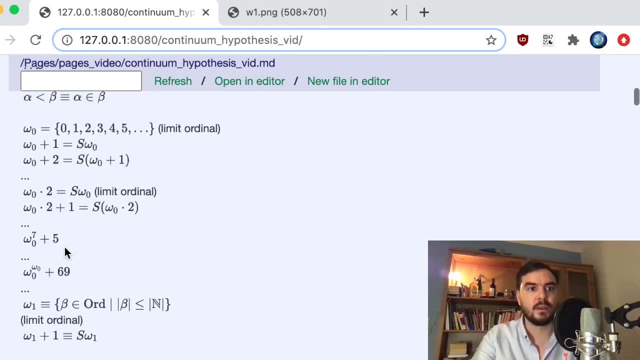 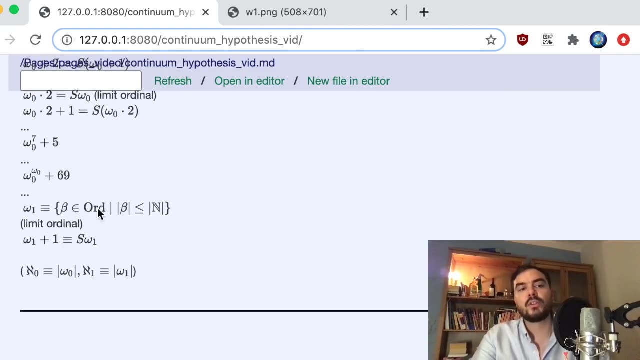 So I have not proven formally that omega one is, uh, is actually an uncountable set. the way defined it, Like I defined it as. let's go back here again. So we said, um, here our definition was all the ordinals that are, uh, finite or countable. 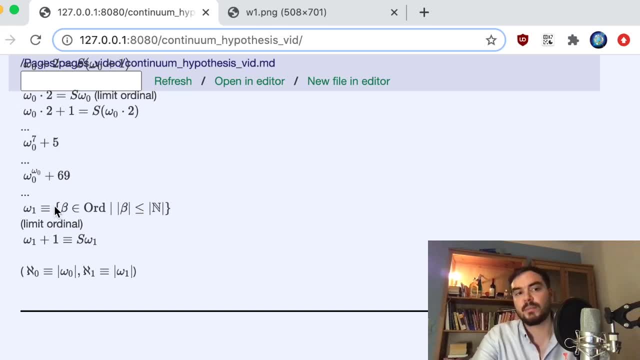 This then turns out to be like, very quickly, uh can be shown. This is an uncountable set, And so omega one has uncountably many elements. If you take any particular element in it, then the left-hand side, so to speak, is uh smaller than the right-hand side, right. 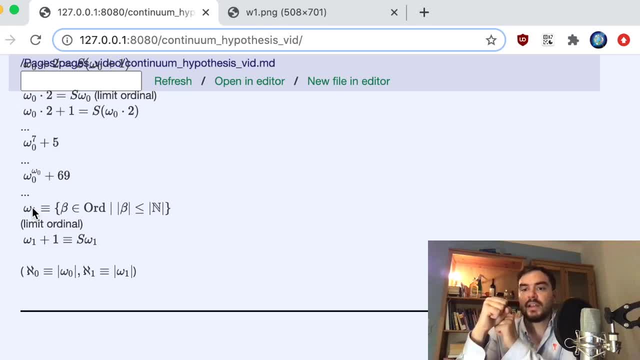 Because, But if you take any element In it, then there's uncountably many elements that are uh, that are uh, bigger than it. right, This is the set itself is uncountable. If you take any element, then on the right side, so to speak, all the elements that are bigger than it, that's, that's always uncountable. 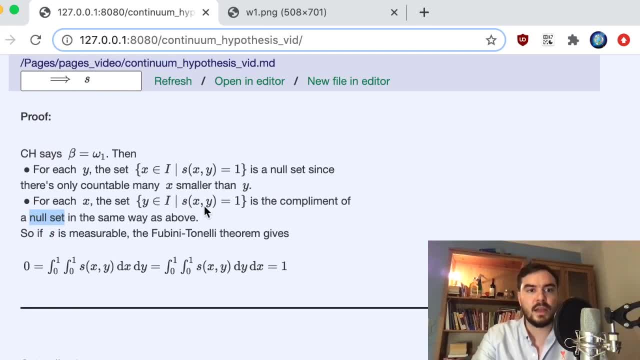 Um, and, and so this is an outset. This is actually, uh, the compliment of analysis. So, Um, if F? S were measurable, then we would have the following: So zero. if you do this integral like the inner integral, uh, for fixed Y over X, then by the first argument here you get zero. 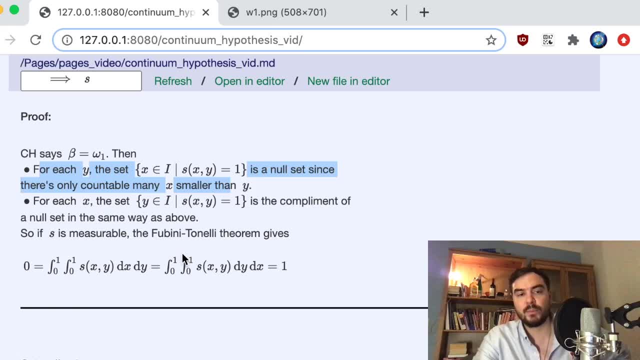 Then, by uh for Benito Nelly, we can switch the integral science right, Assuming the S is measurable. And then, uh, here we get one. Okay, Okay, Because, uh, this is the compliment of the new set in I uh, which has size one. 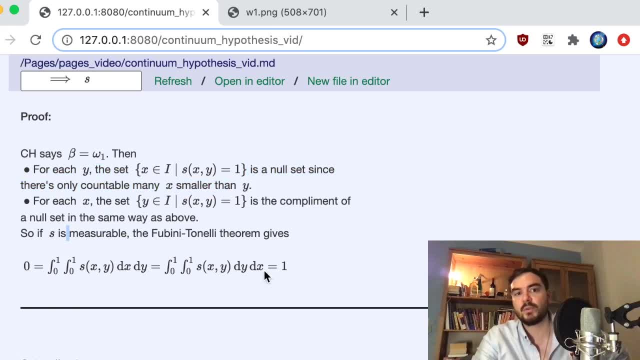 Okay, And so assuming S is measurable, it would give us zero as one. So we find, assuming the continuum hypothesis that S can actually not be measurable, Okay And uh. so I tried to uh to make my hand waving here a little bit clearer with a picture, also hand waving, but maybe you have already crocked it. 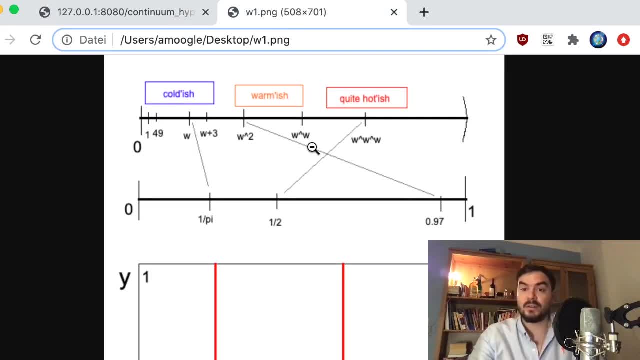 So I have here this, this image, self-drawn by the way, So okay. So here we have um, the, the this top interval, uh, corresponds to the interval. It's basically corresponds to omega one, right? 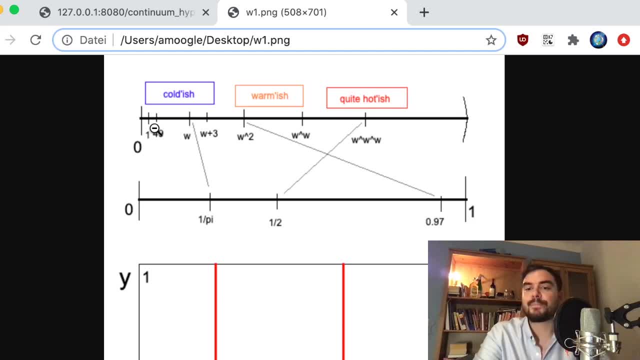 This is the set of all um elements in omega one. So this contains all finite and countable ordinals, Um. it starts at zero, of course, the empty set, Uh, and then it has all the. you know, I I wrote a few. it has one, it has two, it has three, it has 49, it has uh w, here the notes, uh, the omega one. 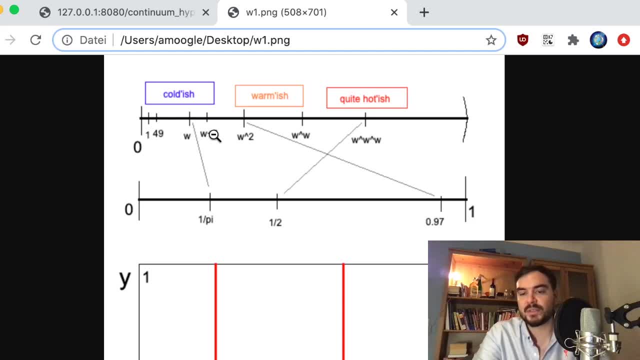 So this is the, the natural numbers, the initial numbers, the three times the successor of it, the national number square like the ordinal natural number squared this ordinal exponentiation here. uh, then omega to the omega. this is what I uh did the video about. 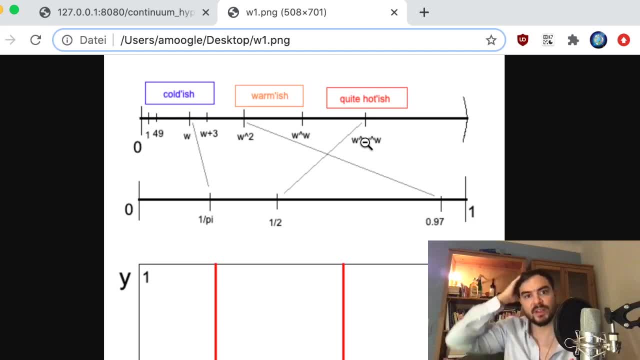 This is also a countable set. You can Go further than that And- and this of course, goes on, There's like much bigger countable, uh ordinals than than just these few examples. Um, but all of these are countable and the totality of them, the, the, the set of those, this is omega one. 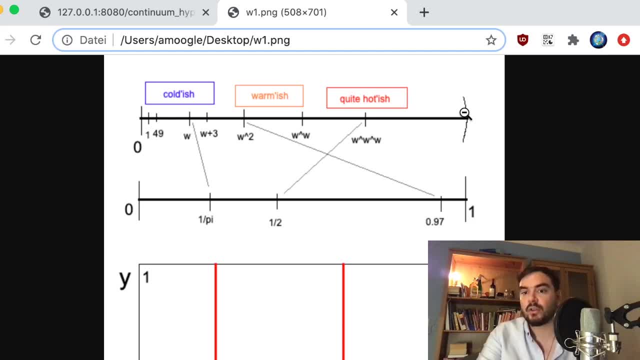 This is what has. um is uncountable And um. if now we assume the uh continuum hypothesis in this, in this hard sense that we have a projection, Um, then to the, this is the interval, the real interval, this is the real number one, this is the real number. zeros. here is is also an ordering, but just a numerical ordering. or here's one of a PI is roughly one third. 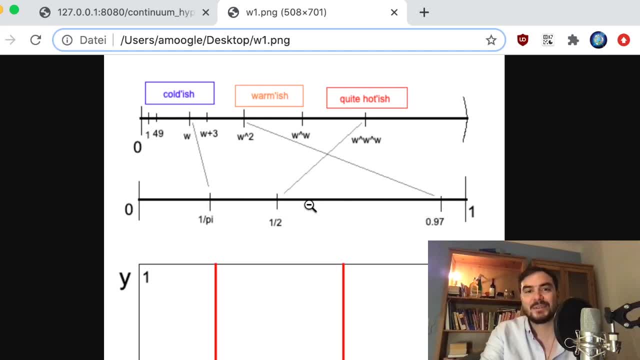 Um, here's one half. it's not really in the middle, but excuse me. then here 0.97 and so on. And this, this is the projection right, This is the B, the correspondence between omega one and this interval. 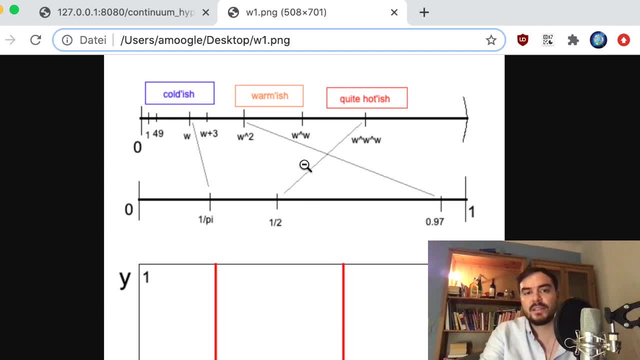 So, and here you. maybe You can be lifted easily. Was that what I said before? Uh, let's pick any element. Let's pick omega to the um, omega to the omega, like omega one to the omega one, right? 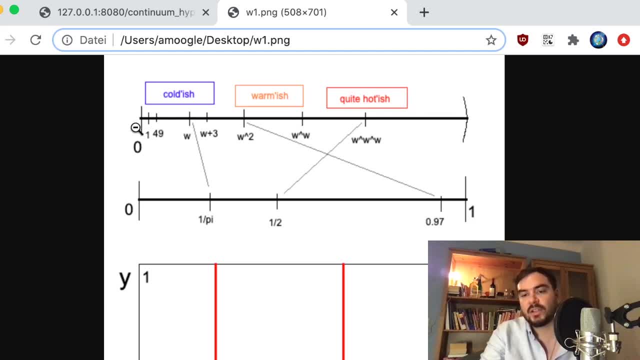 Um, this is a countable or countable ordinance, So you can actually um with uh, you can actually take this set and put it into correspondence, like all the elements here, into correspondence with the natural numbers Right. On the other hand, the whole thing. 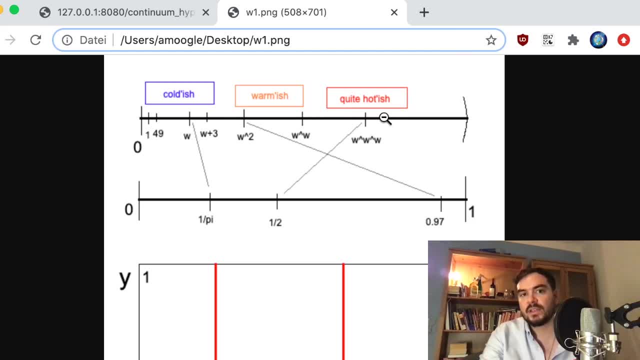 Must be uncountable. So this, uh, in this direction, it it never stops, but in an uncountable fashion, right? So this is uh, in a sense, quotes and quotes denser. the right-hand side is always denser than the left-hand side. 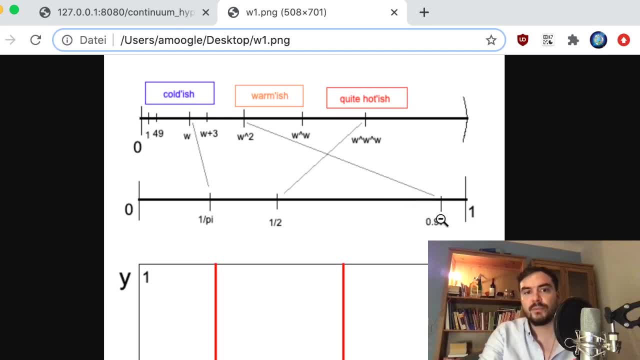 Right. And so for any fixed number, like, for example, if we take this number 0.9, seven, then the, the, the Number of reels that are smaller than this number with respect to the order on omega one, is just this null set right. 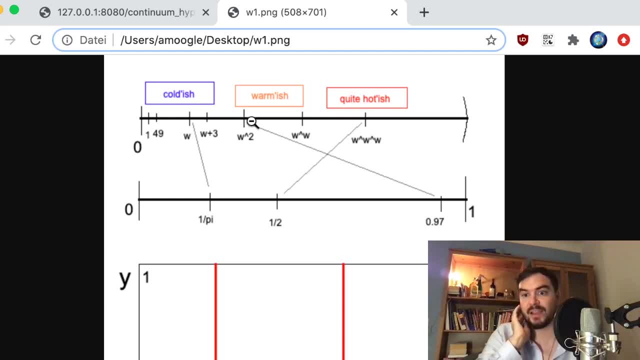 This is just this, this, this natural number, like um, size, um and, in fact, um. yeah, it's easy to understand, Yeah, It's easy to see it from, from uh me, from the other side, like the number of uh elements that are bigger or hotter in my picture, then this number is an uncountable set, because the whole thing is uncountable. 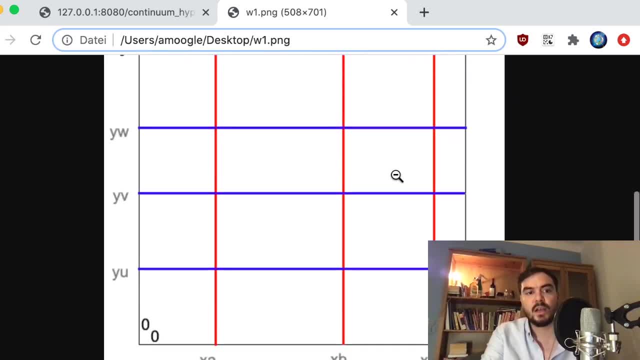 Okay, And uh, so, and, and that's what we see here. So, um, here we have the, the square that we are going to integrate over right With uh for being in two ways. if we fix any, why let's see here then, um, then, uh, the number of elements that are. 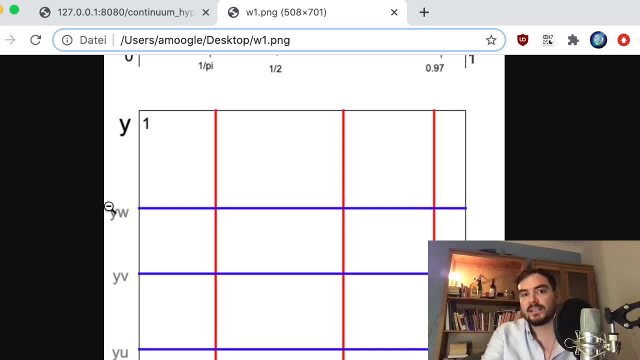 Smaller are these? uh, are this null set? So this is like it's not as dense, It's just. it's just what is here, Um, on the other hand, if, if we fix a Y and consider what is bigger, then this is this uncountable set. 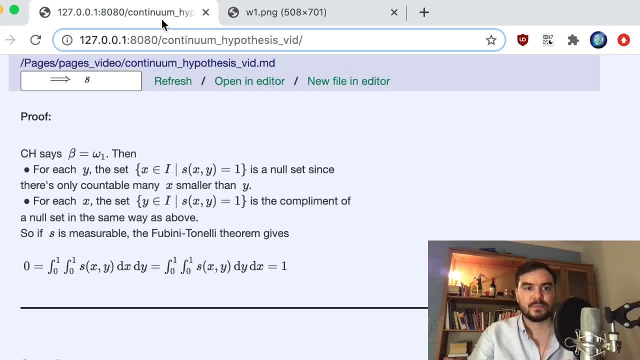 Okay, I hope that uh, that motivates this and this uh continues to prove, of course, uh, you can now uh go on and formalize this a little bit better with actual measures and measure theory, right? 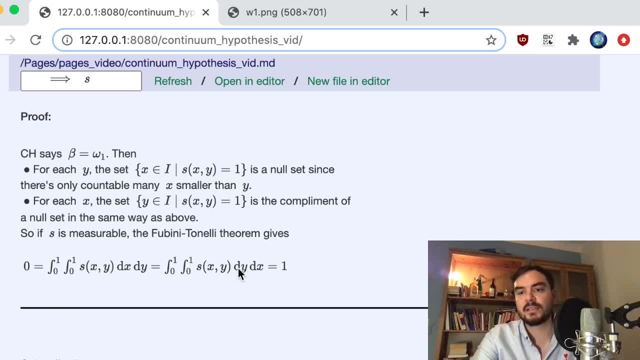 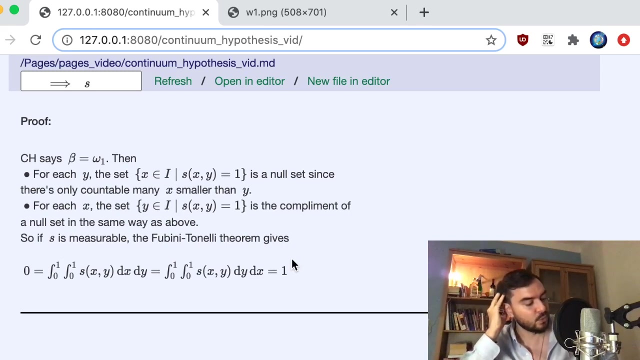 Translate this, Uh, this, uh D-axis, into these proper measures and define actually, uh, these, these sets, um, and, and speak about, uh, their finite and uncountable and um, accountable character, Um, but, as the gist of it, uh, of course, um, if you assume, uh, Tamela Franklin, choice, if you assume the axiom of choice which you may need for. 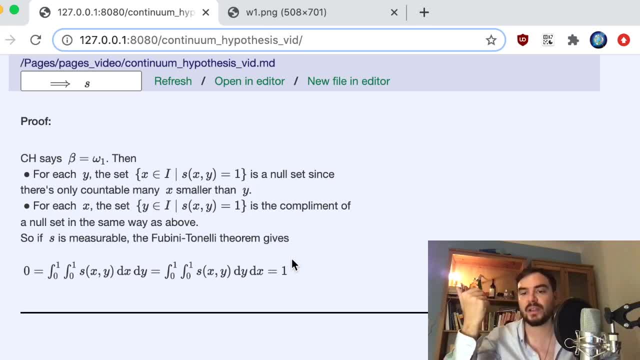 These projections to exist, then a lot alone, but, uh, the axiom of choice there already exists: non measurable functions, right? So, um, this is just a world. If you assume the continuum hypothesis, this then actually implies, um, something which you already had, namely this ugly: non measurable functions. 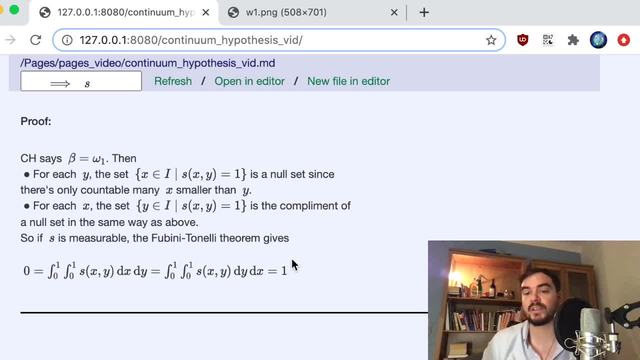 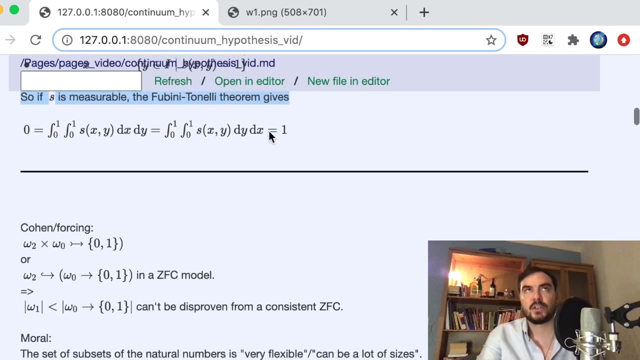 On the other hand, if you add the axiom or if you study the model where everything is measurable, Then this rejects these sort of axioms. then the continuum hypothesis, uh, here cannot hold, because the continuum of offices, as we see here, implies, uh, non measurable sets functions. 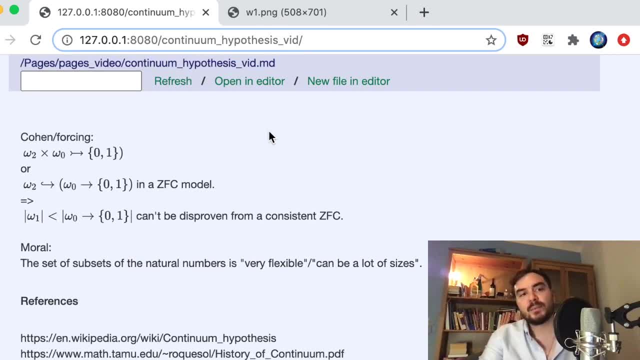 Okay, Um, okay, And, and finally, some remarks. Uh, so this was then, uh, like decades later, shown to uh this conjecture by contour, the continuum hypothesis to be independent of Tamela Franklin choice, even, Um, and, and roughly, uh, the goes like this: there's a bracket too much. you know this bracket. 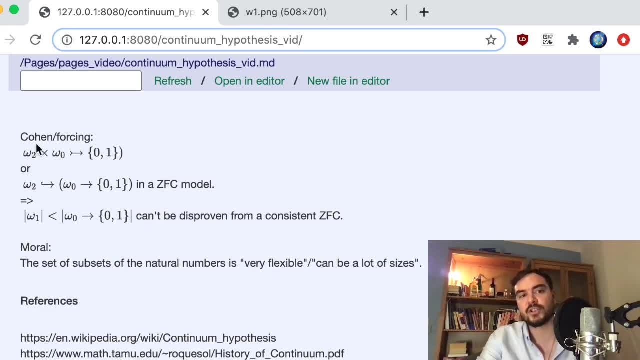 Um, so you, you have uh, these, these functions from omega two times omega one into the, um, into the, this binary, uh set And uh. then uh, you know, with disjunction you had this map into this space. and um. Quinn then finds: 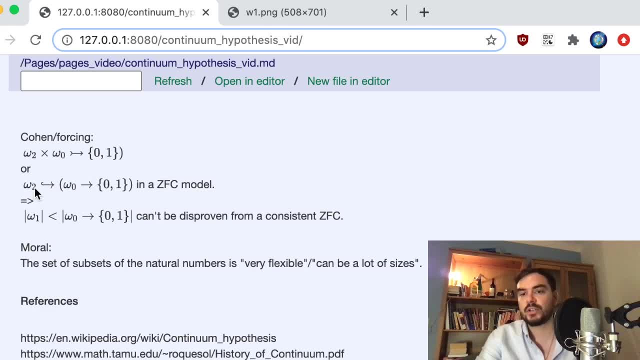 Actually, This injection of this quite large, uh, ordinal, into this object, um, which, which then uh breaks, which breaks then the, the, the, the relation that is conjectured by contour, Namely the, the, the, the power set, basically taking the power set from natural numbers, jumps actually over this. this first ordinal, um, this first uncountable ordinal.